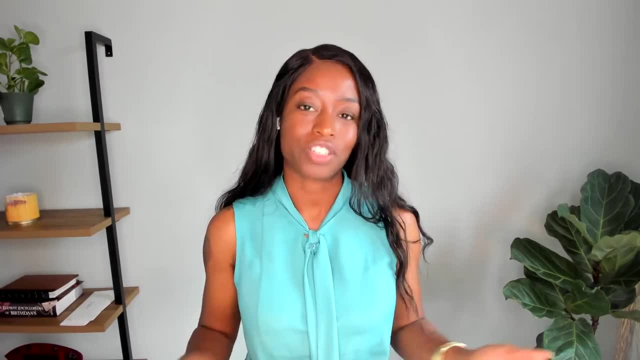 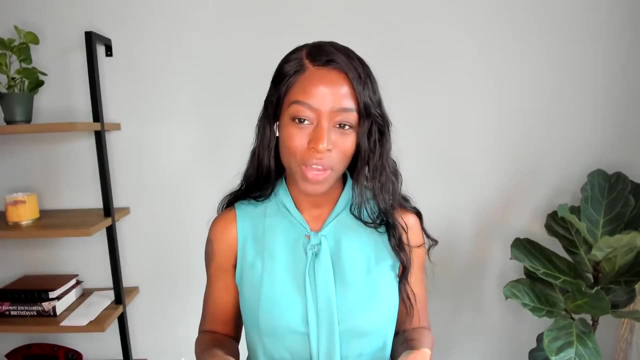 that if you have kids or small kids, you know, in a sense, you're in a new season of life. So one of the things I've seen is that you have to really reframe what a good day is. anymore right, What? what is the? what are your? 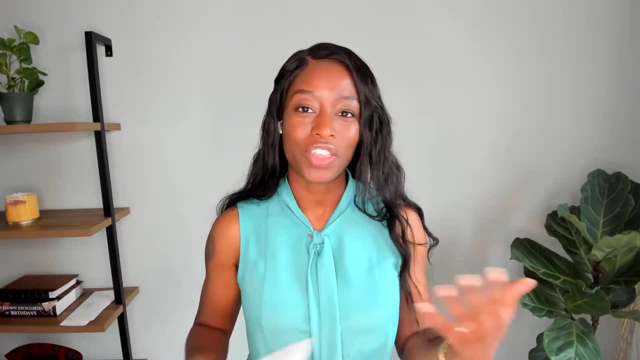 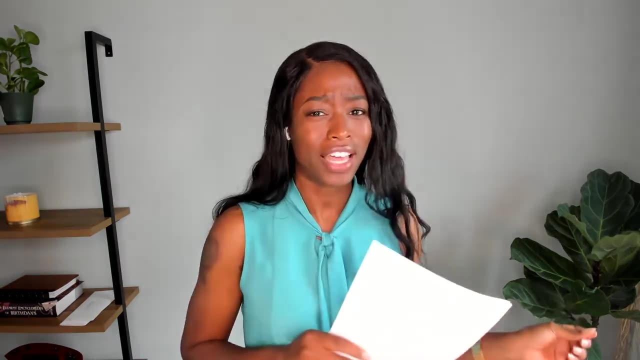 what are your new goals? What are your new, what's your new purpose in life? Like all these things right, There's a lot of catching up that we need to do And a lot of rethinking and recalibrating. that usually doesn't happen, because you're kind of like thrown into this situation. 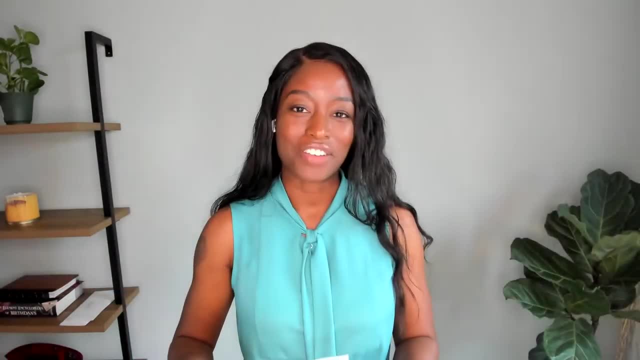 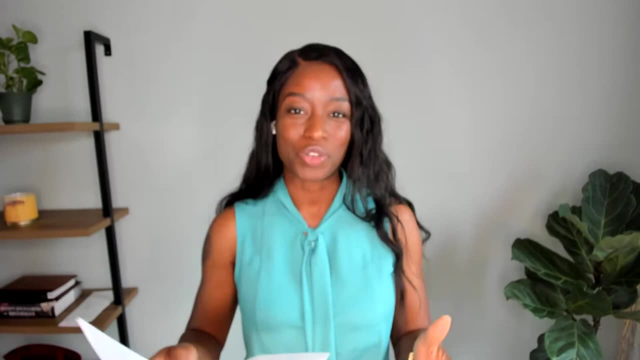 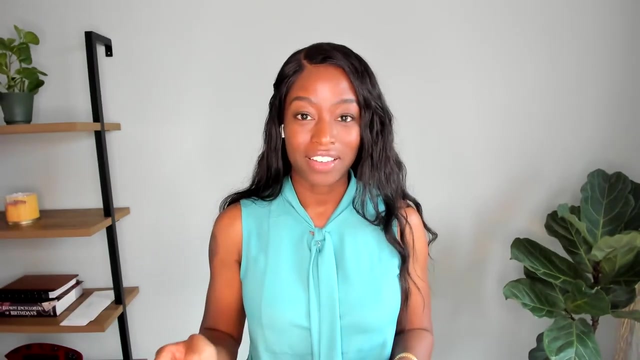 right, You know you are having a kid, but it's like a difference between being pregnant- Now they're here and you're living with them- and having to adjust to, you know, this new person in your life. So the first tip is you have to define what does a good day look like? And then 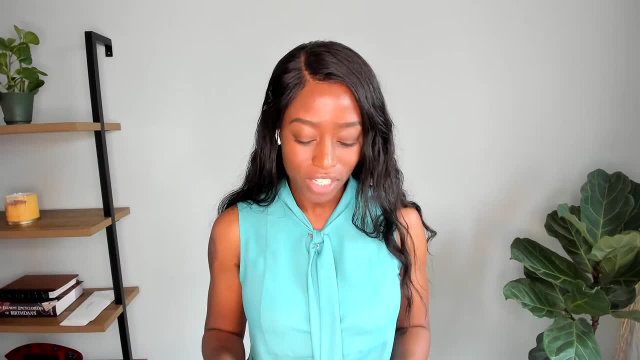 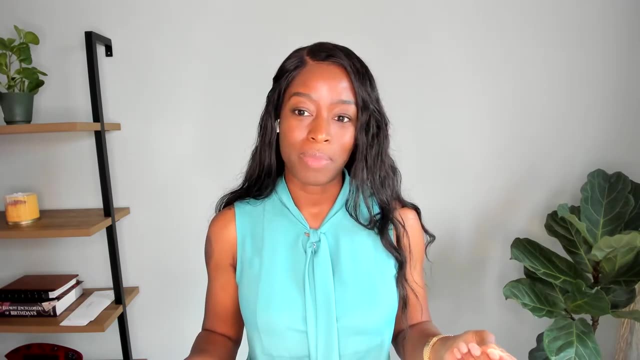 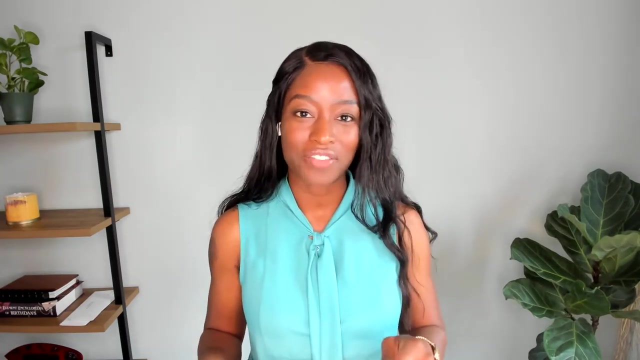 what does it look like in this new season that you're in? Okay, So essentially, if you're used to being able to work out three hours a day and you know you walk around with your to-do list and you're able to knock things off, you know all 10 items get done, you know you're operating. 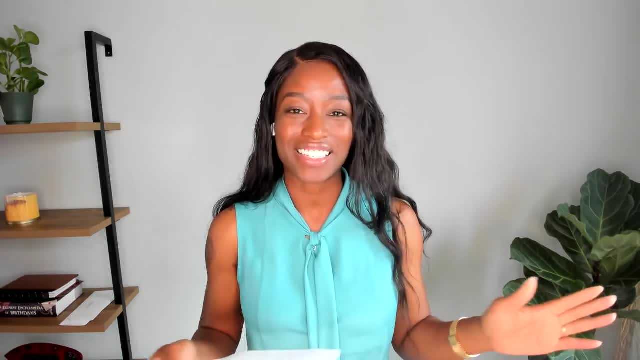 at a hundred percent efficiency and productivity and success. That is a standard that is going to be very, very important to you. So if you're able to work out three hours a day, and you're able to work out three hours a day and you know you're able to work out three hours a day and you're able 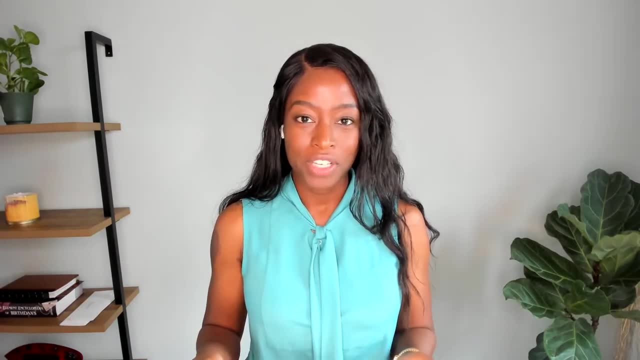 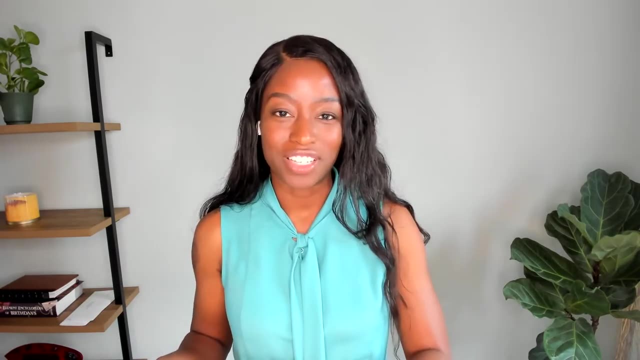 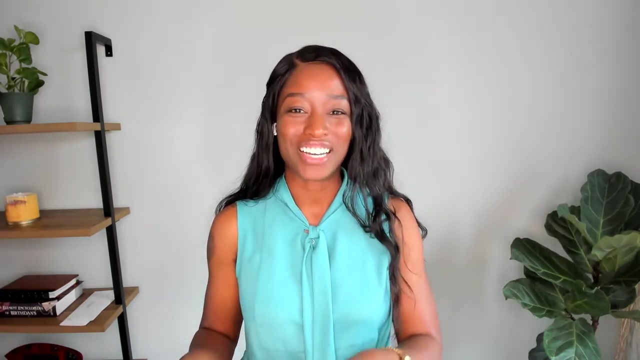 very hard to achieve with your small kids. Okay, So now a good day may be actually getting into your shower and your body washes there, right, Like that's a great day. And it's like, oh my God, I'm so excited I have body wash in here. You know, I don't have to go to anyone else's. 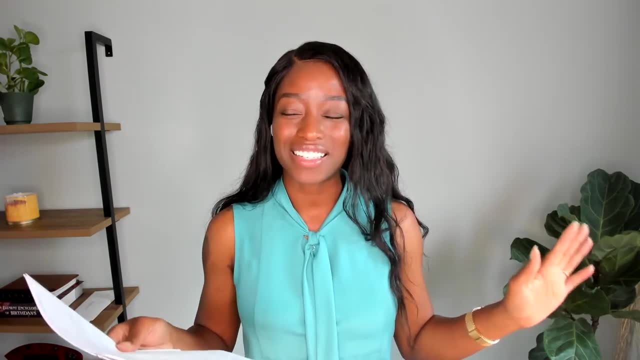 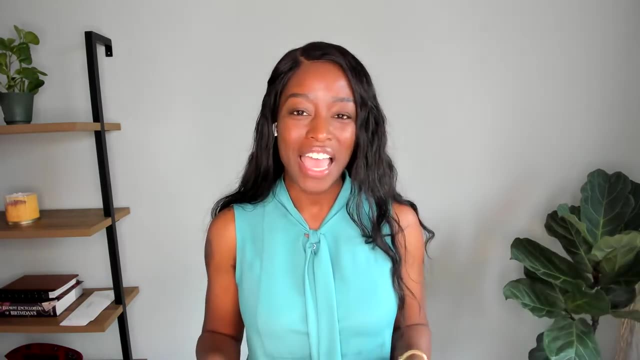 bathroom looking for it. Nobody stole it Like, yes, yes, yes, I'm on top of the world, Okay, Um, another way to reframe it is: let's say, you have this huge to-do list and, um, you know, you come, uh, downstairs and you know it's one of the kids they're not feeling. 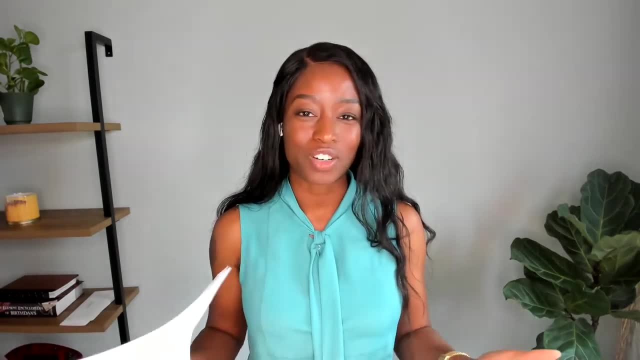 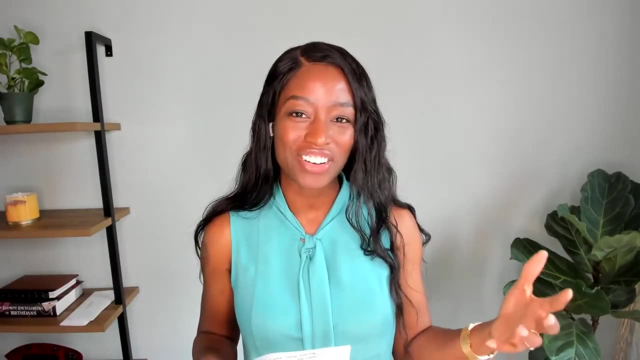 too well or whatever, And you can tell they really just want to snuggle with you, right? They just, they just want your scent, They want your love. It just is what it is. but you've got this long to-do list right here in your hand. You know, glory is so close, right? You dreamt about all. 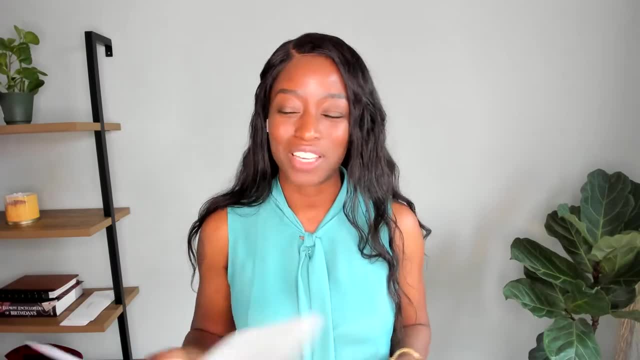 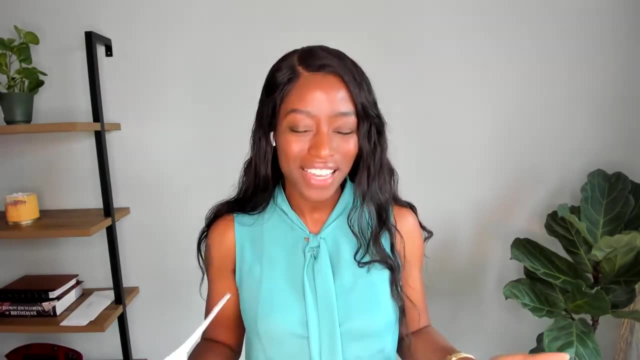 the things you'd be doing today, And again checking off those boxes. but you've got the kid over here, That's. you know. like I said, they're looking at you for once. They actually look really cute. They look kind of pitiful and it's like you know what. Okay, I'm gonna sit down. 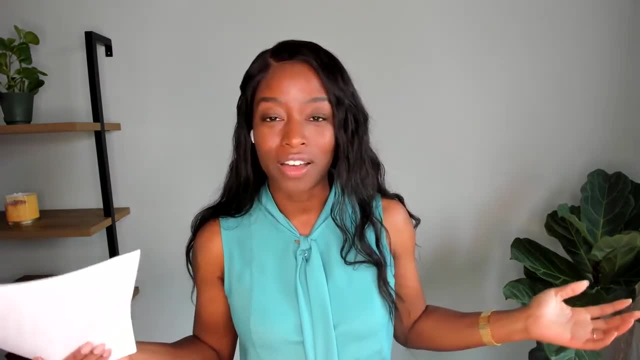 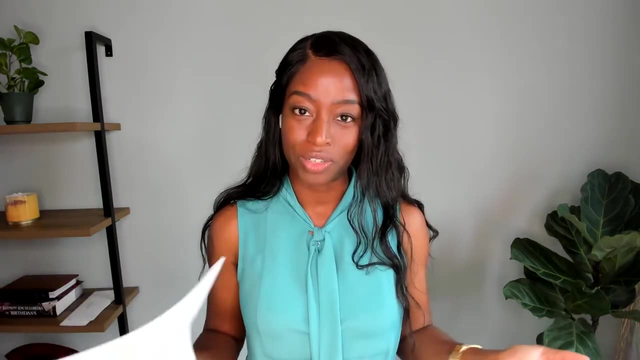 here I'm going to give them some love. Well, that turns into the whole day gone, right. How do you view that day Right? Did today suck because you didn't get anything done on your to-do list? Um, did today suck because you had to sit with that kid all day just holding them? 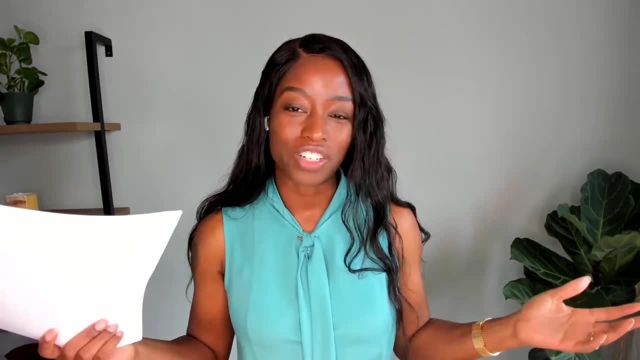 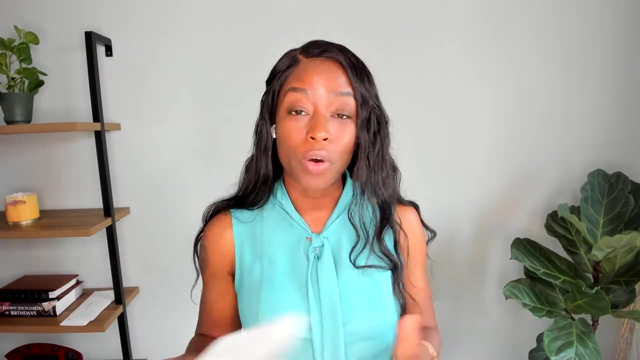 there, um, while they, you know, watch TV or did whatever mindless thing that kids do. I don't know what goes on in their heads, but, um, or will you consider that a win, right? Because you got to sit? 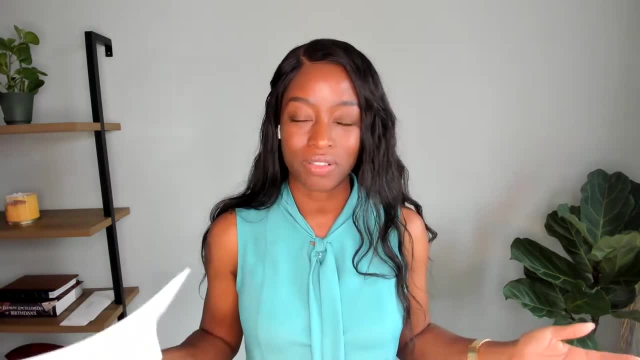 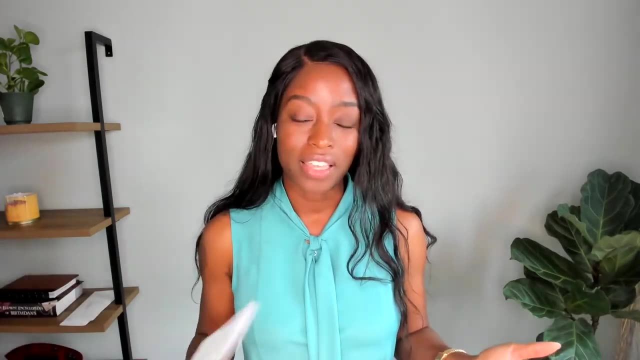 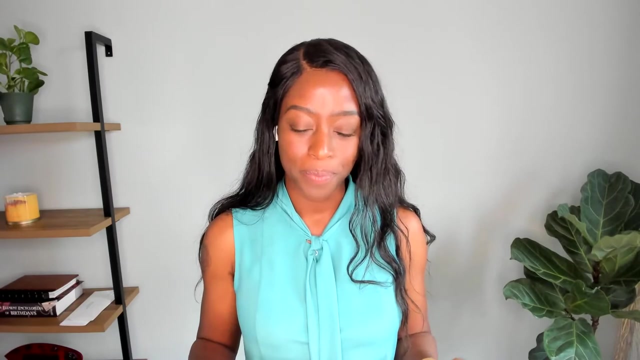 with them, nurture them in that moment. It is what it is. Tomorrow's a new day, Okay, So hopefully you see where I'm going there. that your perspective on what is a win in this new season of life It. you may need to adjust that to where you currently are. Okay, It's a new season, It's a new day. 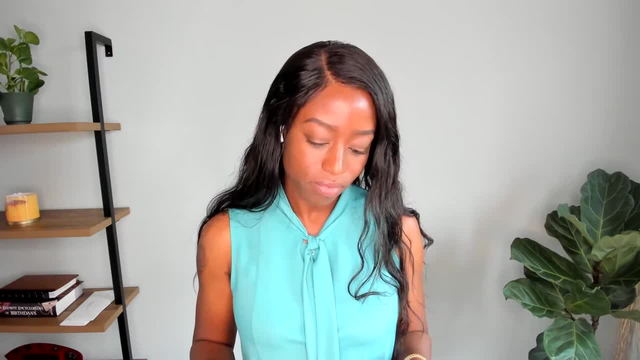 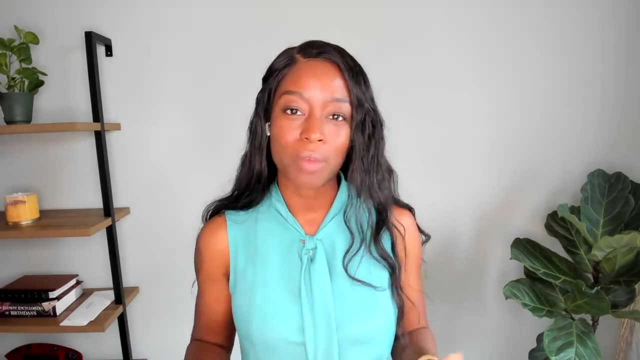 Okay, Um, let me see. So, yeah, if we're in this new season, it's going to be really hard for you to do things like keep the house clean If you're still operating as though you're in the old season, whatever that. 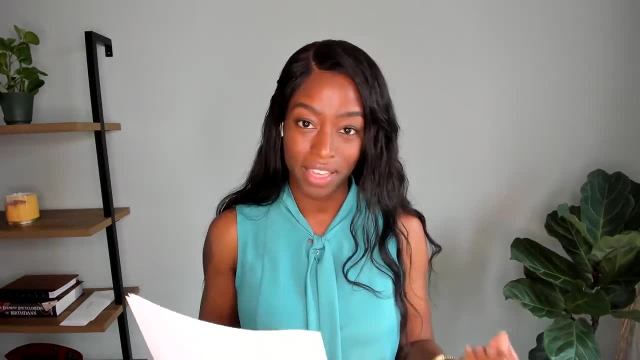 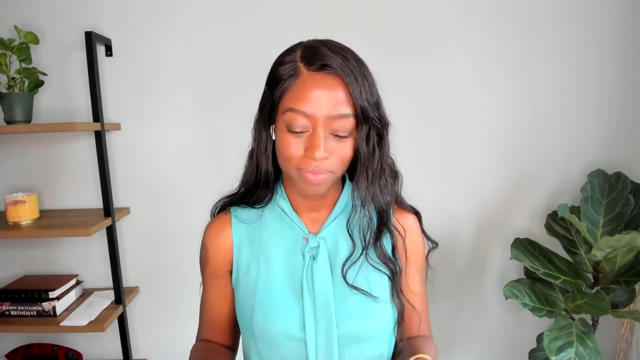 may have looked like it's going to have to change. So that's the big thing. Okay, You need to reframe. what does a good day look like now? Okay, Next tip number two is be prepared to let some things go. 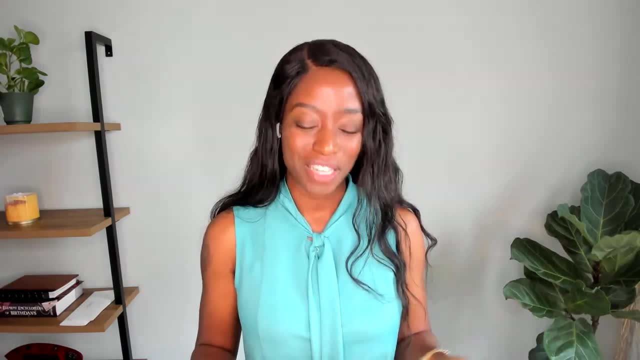 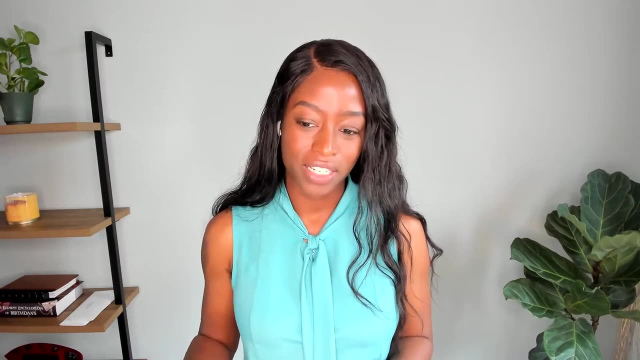 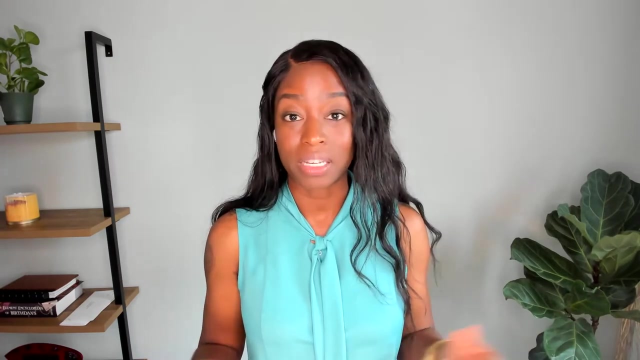 So it kind of piggyback piggyback. excuse me off of the first tip, but with that one it's um some certain things that you realize. all right, you've got another person in the family or you've got the three kids, and it's a bit much right. So I guess number one 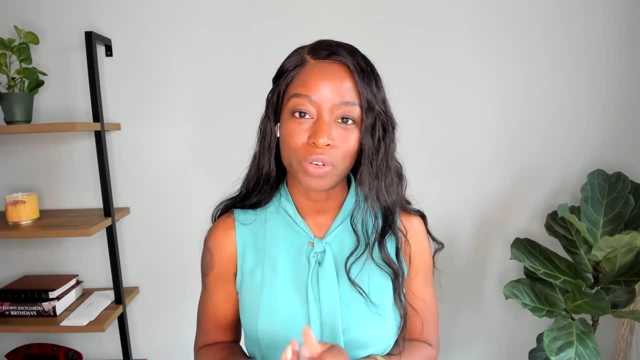 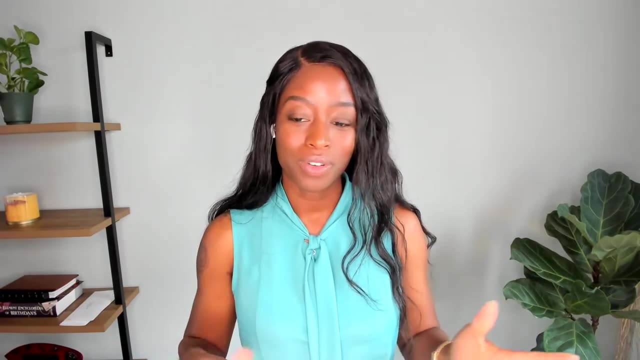 you have to be honest with yourself. This is a bit much. I don't feel like I'm doing very well. Um, now look at your life. What are some things that you like? I said I mean, your plate is full. 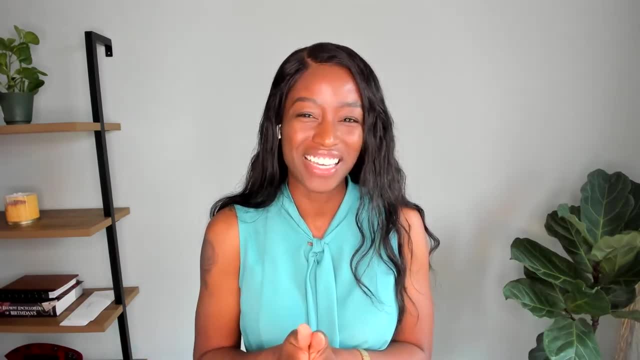 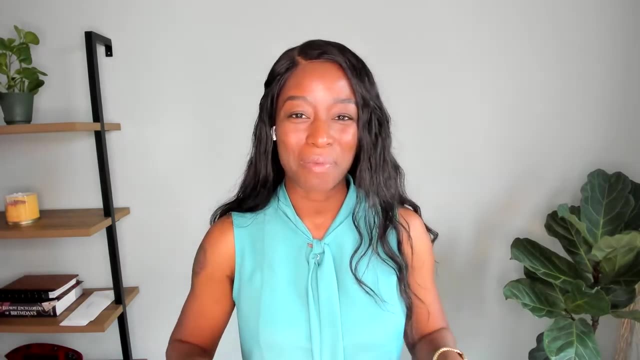 All right, And I'm hoping the kids are are a priority. So if we say, Hey, you know, we know that they're definitely staying and you've got a few other things that we definitely know, Hey, I'm not, you know, letting these go, What? 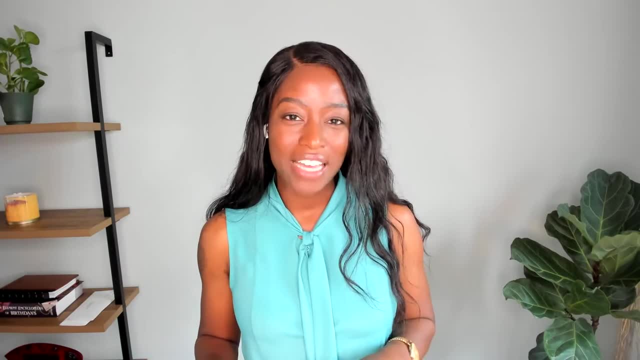 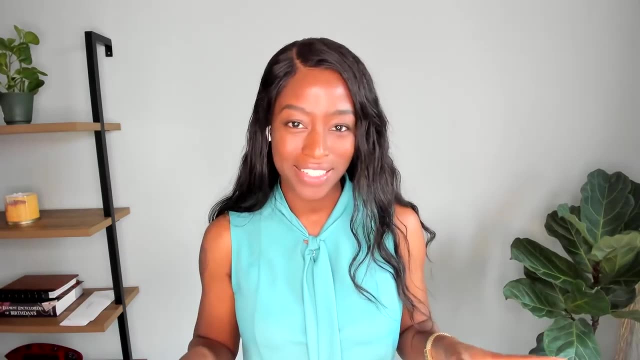 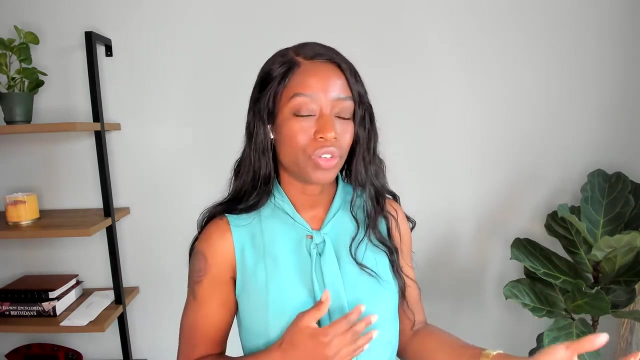 can go. So sure, You may have had three dogs, you know, before you brought in the small kids, but now you've got three dogs and a baby. That's way different, right? What about with two dogs? make your life easier instead of three- And I know that's hard to you know, manage. but 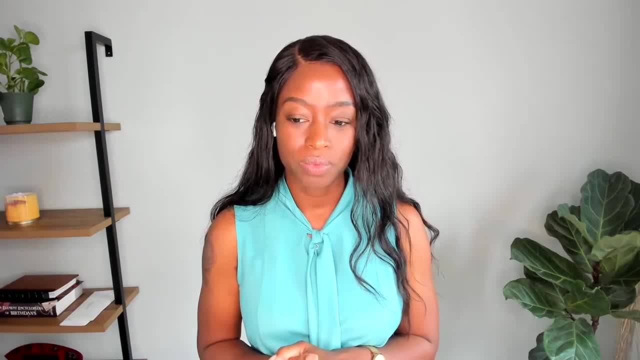 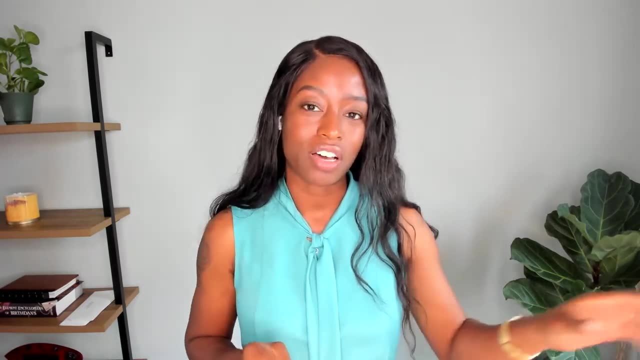 think about it this way: You, if you're operating on zero cylinders, you know, and you're kind of giving your half best, half attention to the dogs, half the attention to the kids, half your attention to work, half your attention to projects, your, your partner. 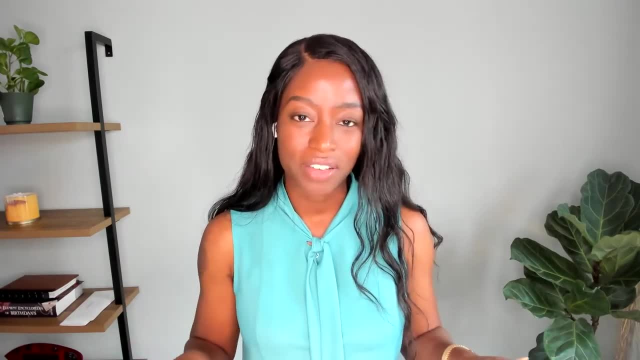 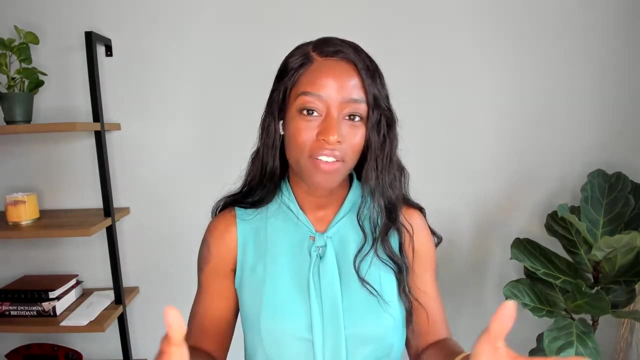 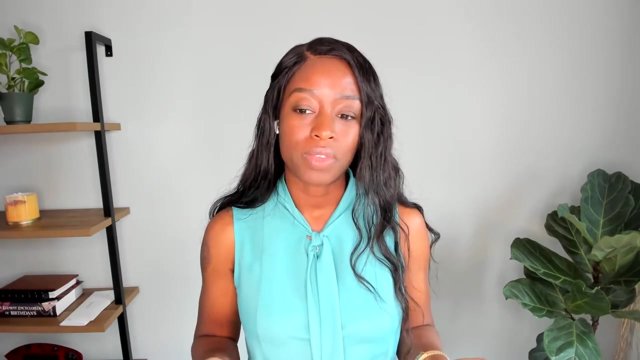 you know all of these things are getting half of you, not the best of you, is what's the point then? right, Um, when you rather have people in your midst or things in your midst that you can give all of you, to give your a hundred percent best to. So if you're stretched thin, then you're a. 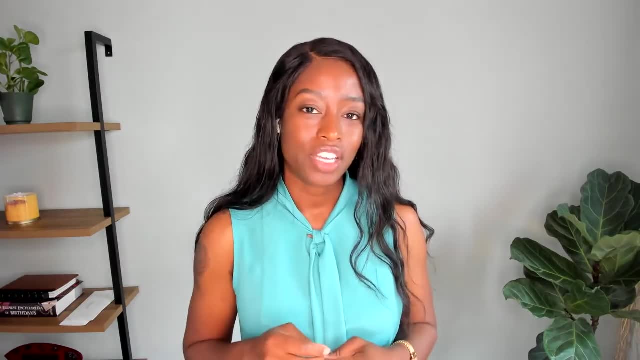 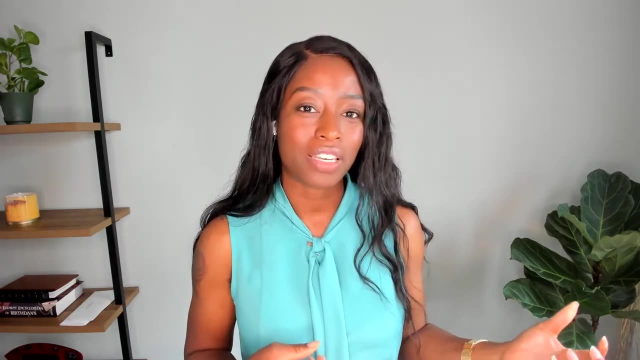 mother that's stretched thin. You're a partner that's stretched thin. You're a? um, a fur baby mom, I think that's what they call them. You know that's stretched thin, which means you're probably not the mom that you want to be, or you're probably not the partner that you want. 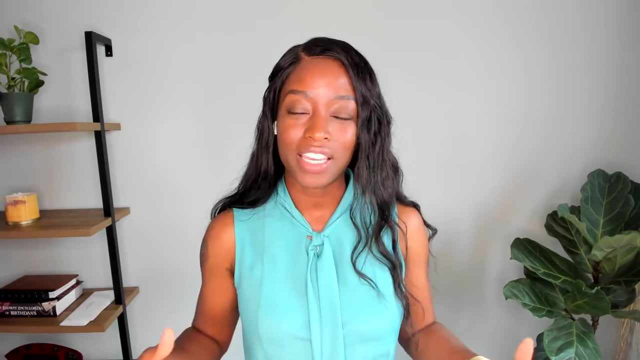 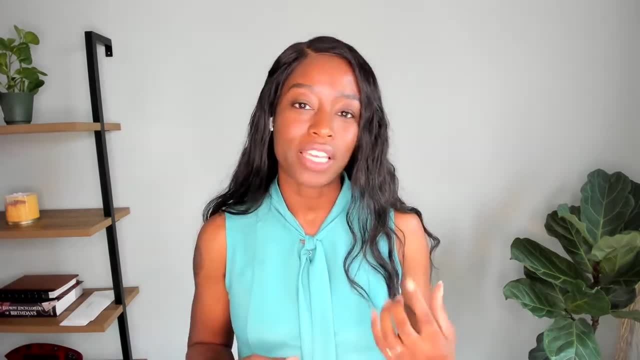 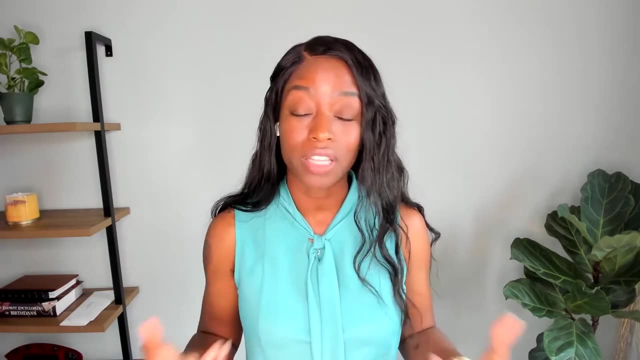 to us because we consider them either a part of our identity or, again, you know we do love them. But again, when we're not able to give our best or show up in a way that we need to, sometimes the most loving thing you can do is to let those things go, All right. And I say all that so that 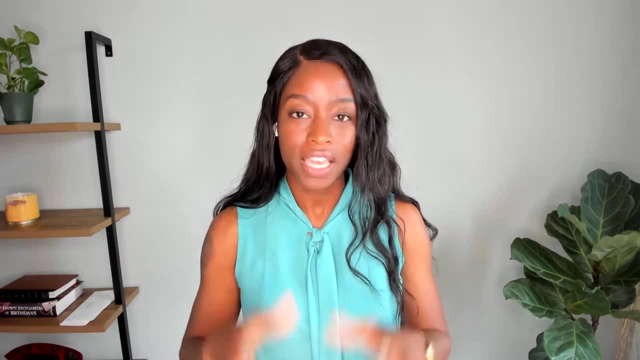 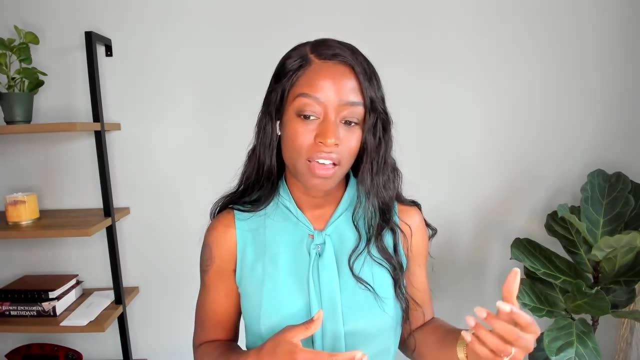 you can make space for whatever you need to bring in in this new season of life so that you can operate at a hundred percent. Okay, So maybe you do need to let the the um dogs and cats go, and that will give you the space to let those things go. 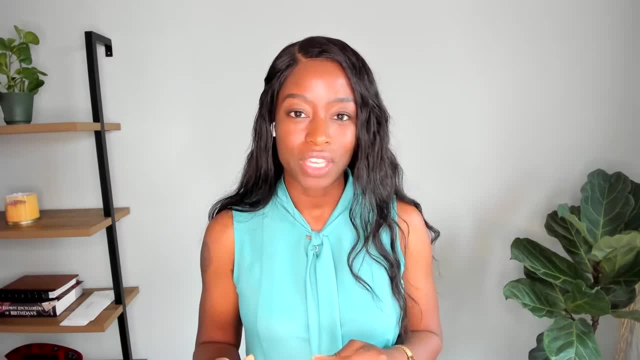 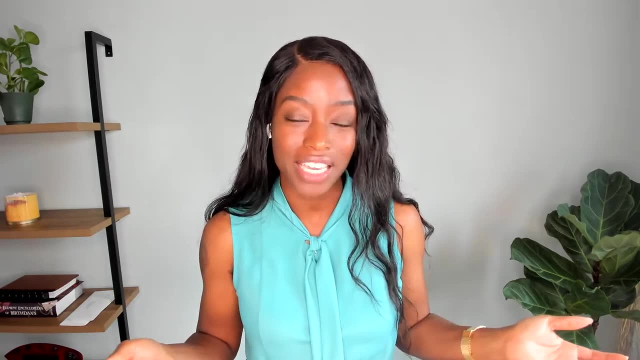 More mental space and more time to do things like um meal prep. All right, Maybe your health. you're noticing that you are putting on some weight here, right? Some stress eating. So look at things from a more holistic perspective. take a step back. You know you have to be a 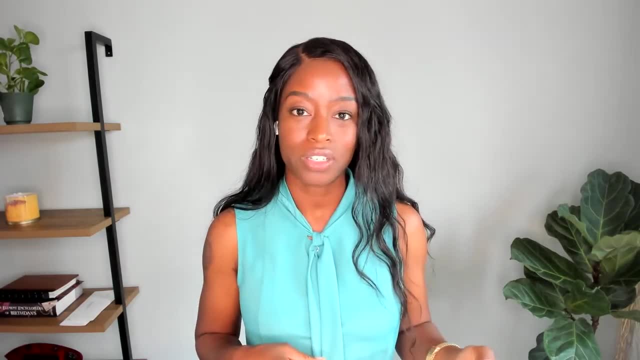 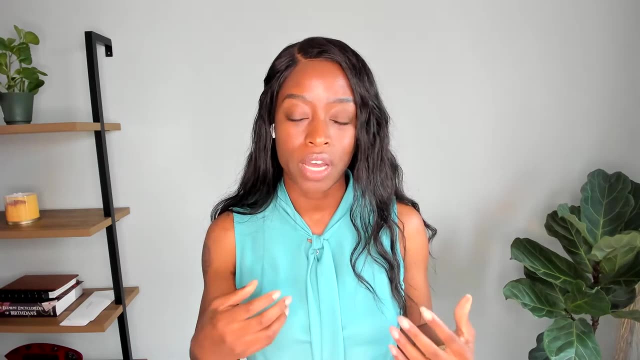 little bit more pragmatic. Everything can't be an emotional decision, So to speak. you need to think about things, um in regards to, like your, your legacy. you know purpose, your um being responsible versus irresponsible. you know all those things And those are. they're tough, You know. it does require. 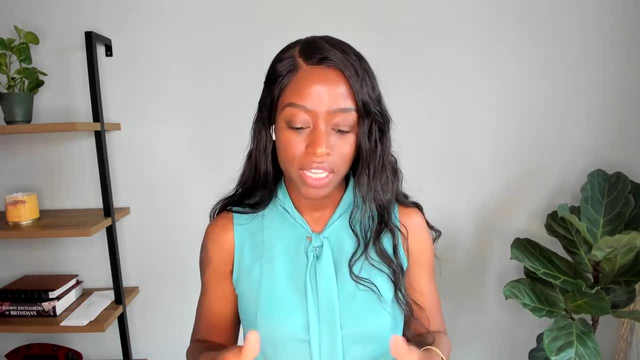 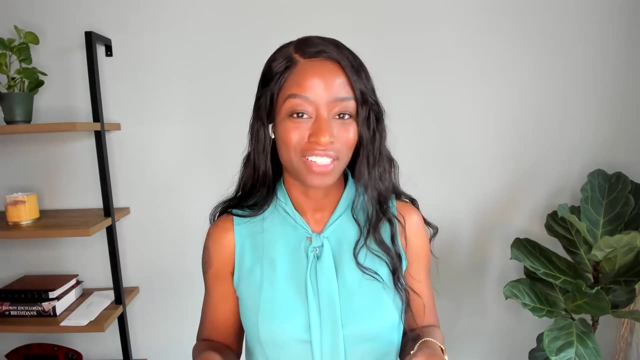 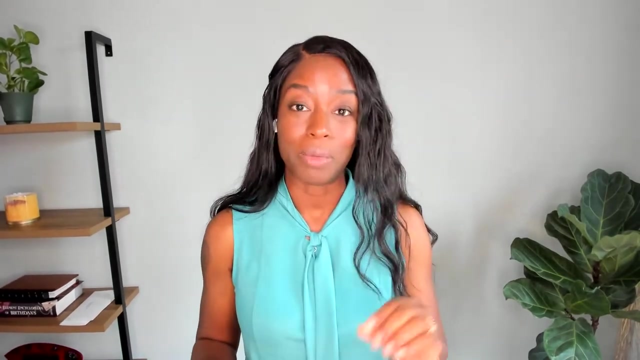 a bit of self-awareness. but again, it is necessary in this current season of life because it's a tough one, and it's hard when you're operating, you know, on half cylinders. you need all your cylinders to make it through this season. Okay, So let's move on. Well, be prepared to let. 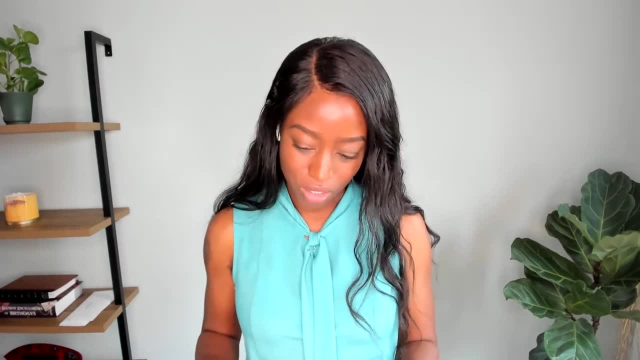 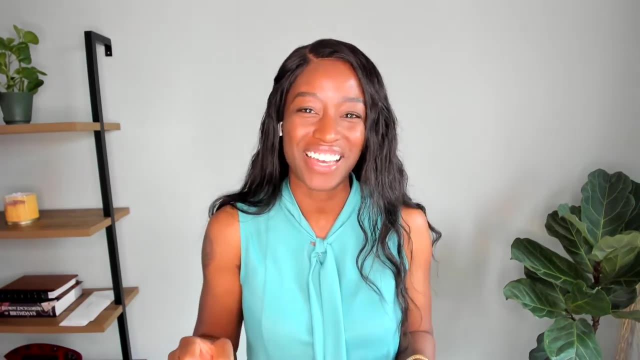 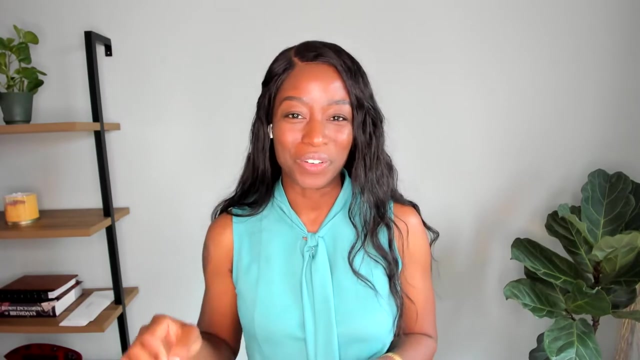 some things go All right. That was tip number two, So let's move on to tip number three, And that is, you need to understand where your kid's brain is right now. Okay, So we're talking about truly understanding that. Yeah, You need to know what they get and then what they don't get. you know, uh, certain. 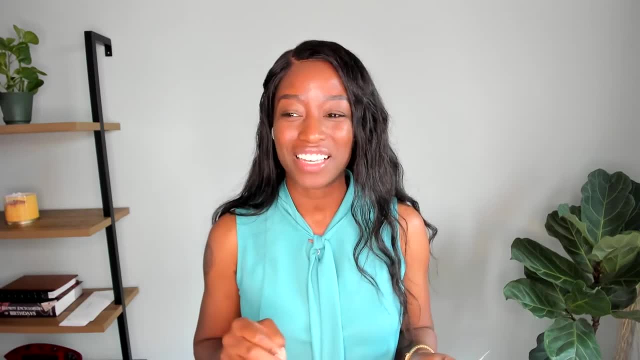 things are going to tick them off. So if they're playing and all of a sudden you say, Hey, it's time to go, Hey, they're ticked off, They're going to explode, All right, And it's because you didn't. 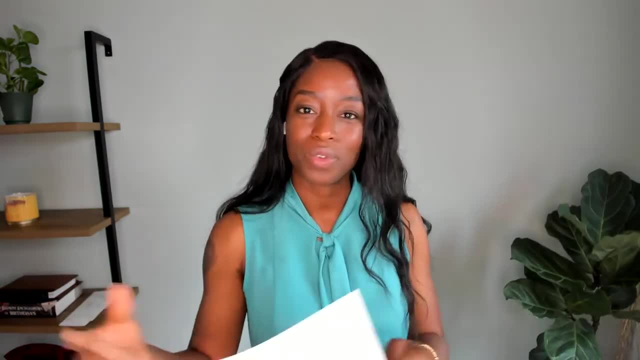 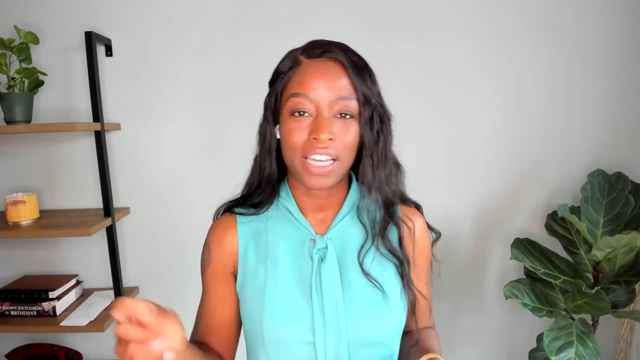 give them a heads up and enough time to, like, mentally, transition out of whatever activity they're in until the next Right, And you can't be mad at them. You can't be mad at them until you're at them. It's not a thing of, hey, I'm your mama And I said: do this, And you're not moving fast. 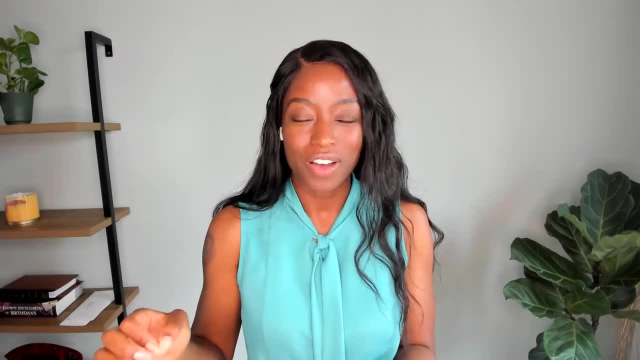 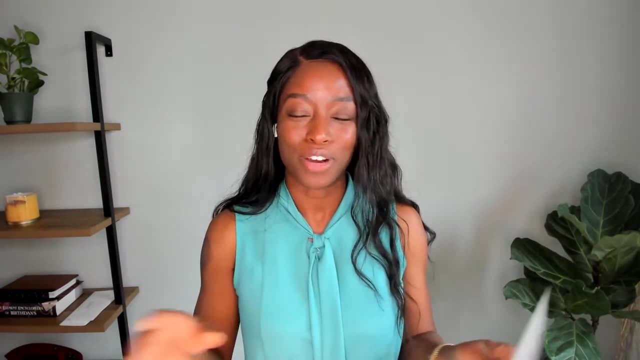 enough. blah, blah, blah, blah blah. No, their brain, like the chemicals, the neurons, the synapses and all these things, they are firing off And right now they are out of state in their life. Their brain is well, I don't want to say underdeveloped, but they're not firing off on all. 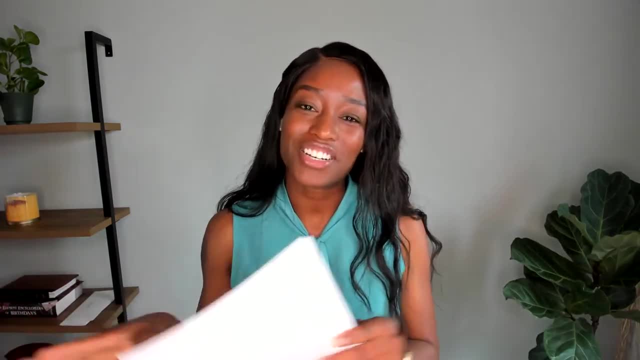 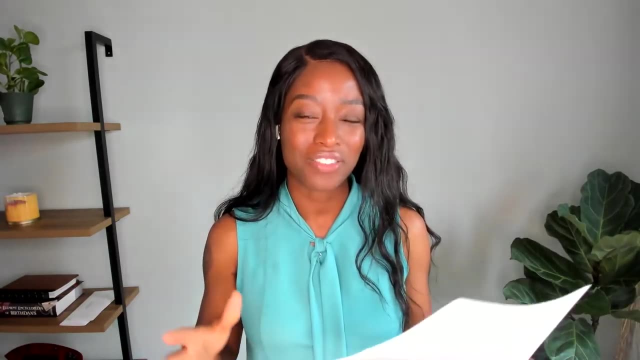 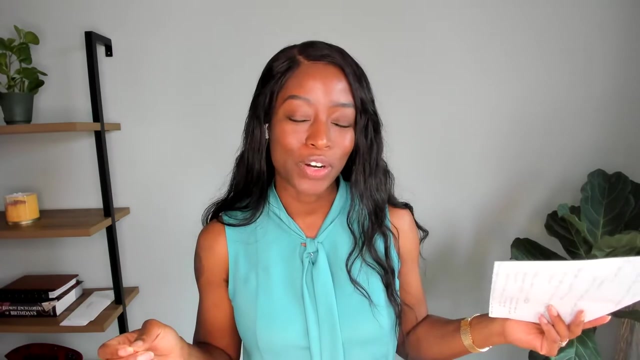 cylinders just yet, Or we'll just say you might have 10 cylinders. Your kids only got one right now. Okay, So you have got to be a little bit more understanding of literally where they are in a neuropathic sense. I don't even know if that's a word, but you get what I'm saying. You guys are. 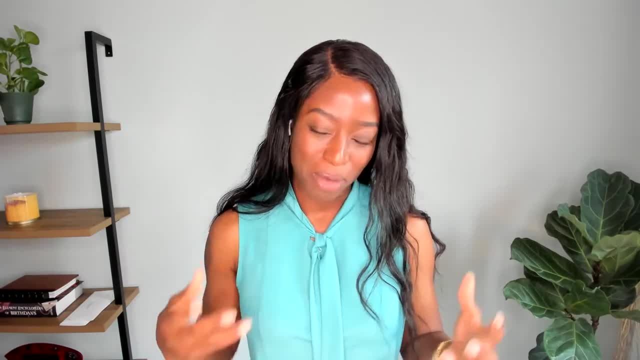 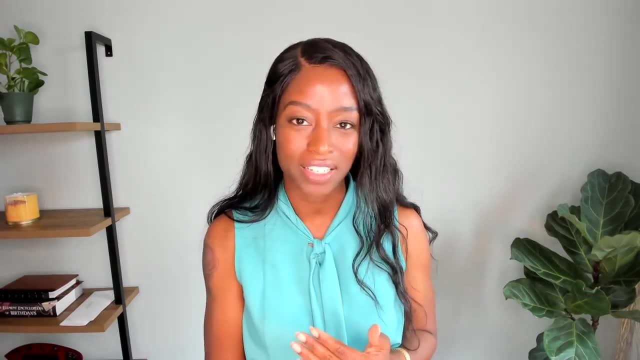 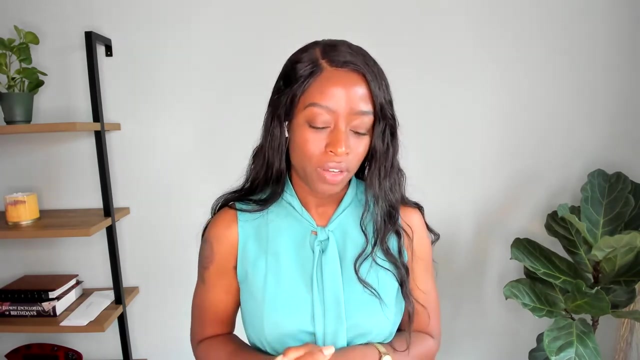 smarter than me, So you understand. It's about being age appropriate, developmentally appropriate and your expectations of them and how you communicate with them. Okay, That's a very big thing: How you communicate With them. So, with that being said, um, the kids: one of the things I realized is that they need 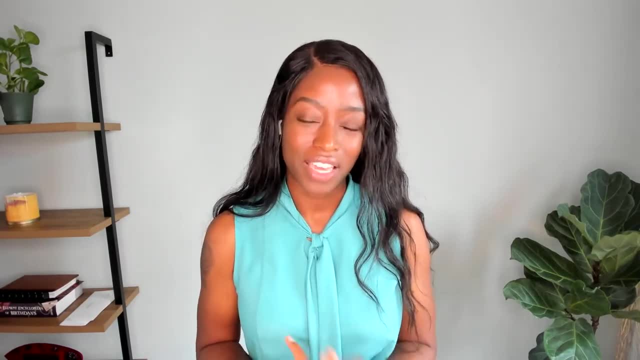 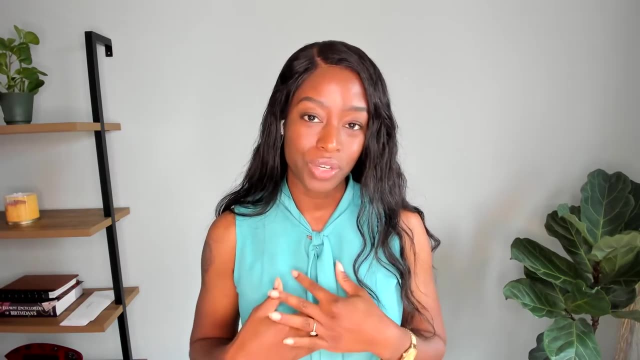 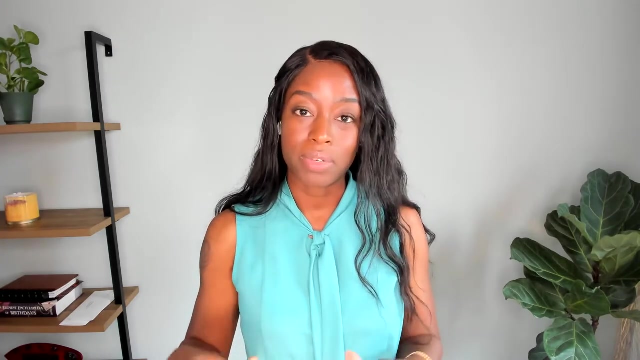 structure repetition and lots of heads up. Okay, Structure repetition, lots of heads up. So that requires you, as the adult in the house, to make sure that they know. Hey, um, you know, this is the play area. When we finished with the play area, this is what we do. I'll give you a. 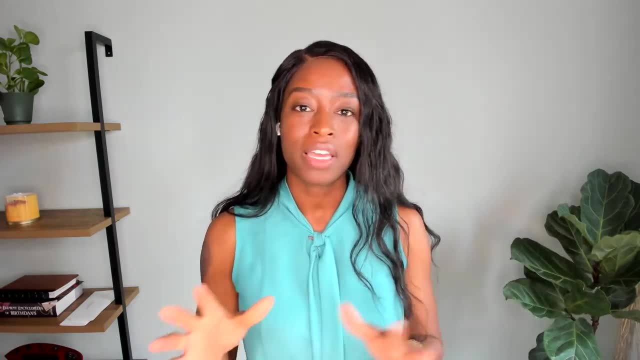 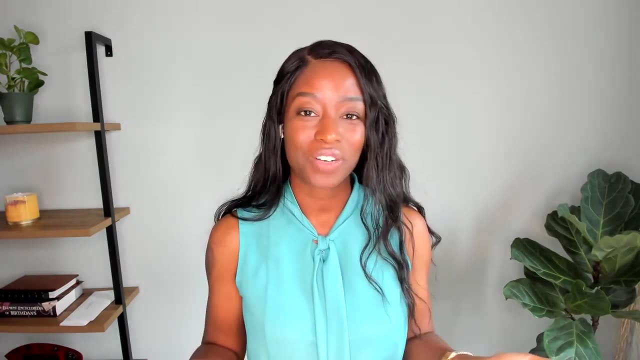 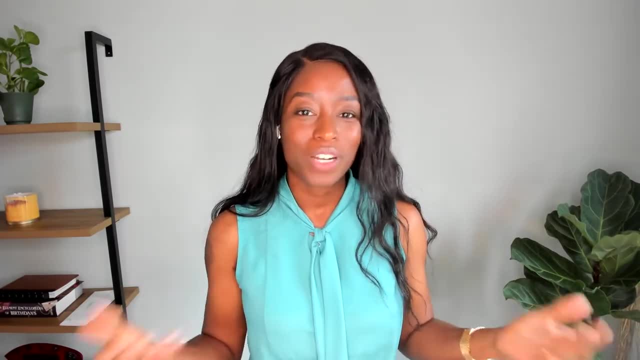 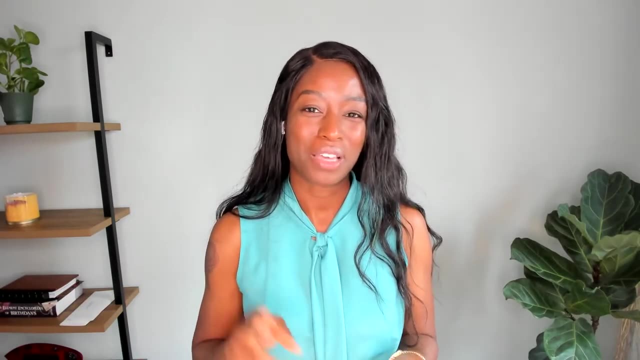 night, when I put my kids down to bed, I always ask them: Hey, what are we going to do in the morning? We're going to wake up. We're going to brush our teeth, wash our face, put our clothes on, eat our breakfast, put our shoes on, put our jacket on, get in the car, get to school. 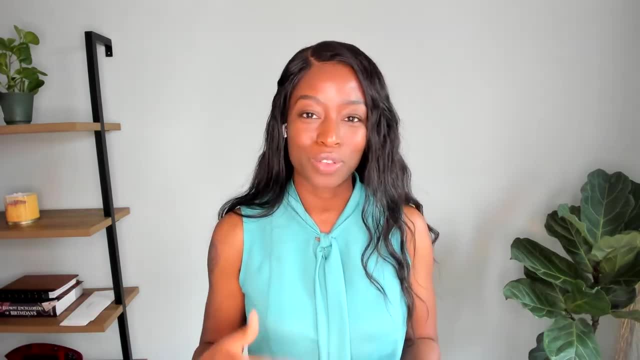 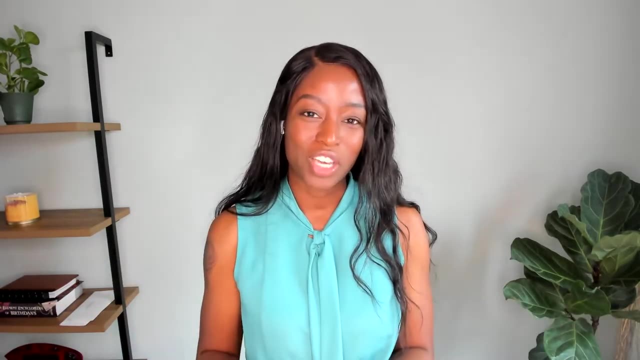 have an awesome day, Right, And I literally, we literally run through this every single night. Hey guys, what are we going to do in the morning? You know, boom, boom, boom, boom, boom, boom, boom. And this has made our mornings go so much better, because they literally wake up, you know, and 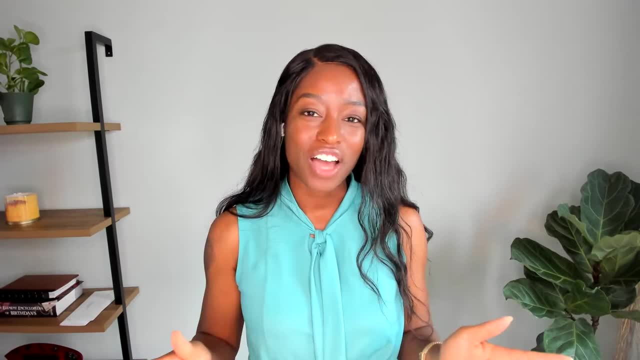 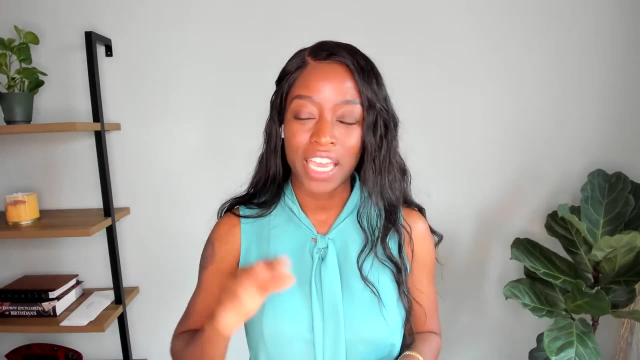 they're doing you know the things right And they feel accomplished, They feel good as opposed to, let's say, there was no order, Right? So some days they get up and I'm like, yeah, uh, here's breakfast And they're like, Oh, what about brushing our teeth? I'm like, ah, whatever. 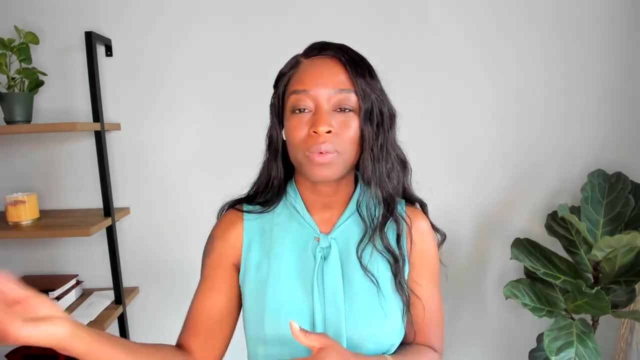 just come eat your breakfast, And then you know they're like: okay, well, now we want to watch TV. The TV was on, And so now I'm like: Hey head up, Get your clothes on and all this kind of stuff, And then it's just chaos and everyone's falling. 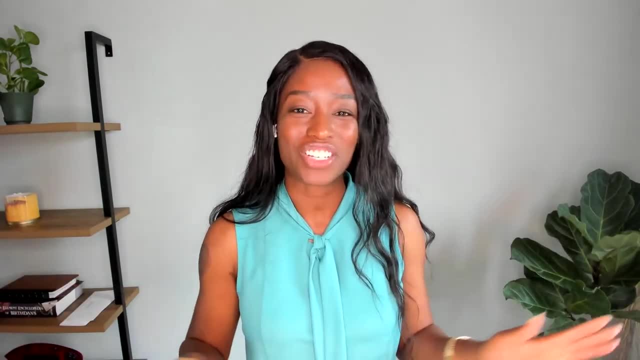 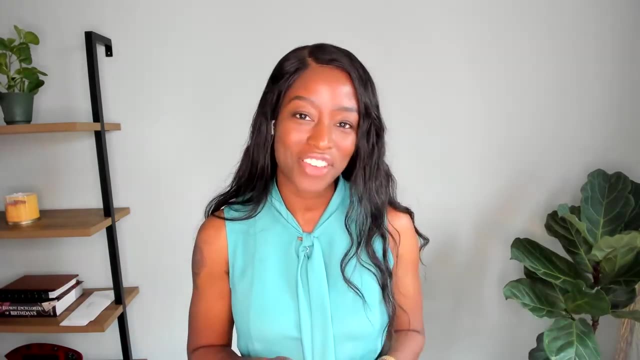 apart and it is not a good day And that is not how anyone should start their day, Right, Whether the kids are going in. let me rewind: My kids just started going to school, So this has been a long five years because it was just me and them. I'm only even able to make this video because they 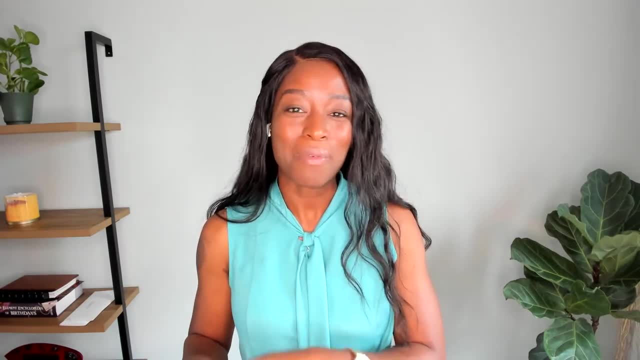 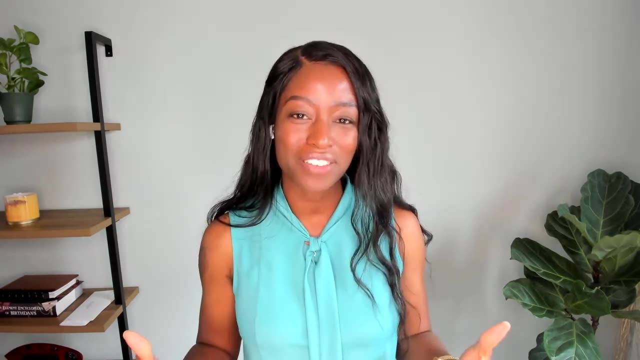 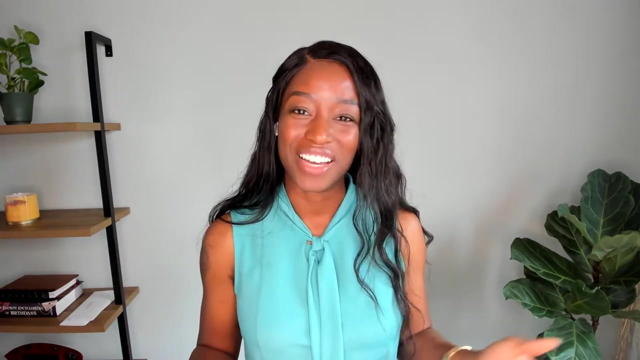 are all in school and I only have like 30 minutes left before I'm going to have to run to go pick them up. So, anyway, just trust me, be this, this, this perspective, It's my own and it is battle tested and proven. Okay, I'm able to still smile. I do not have tears. 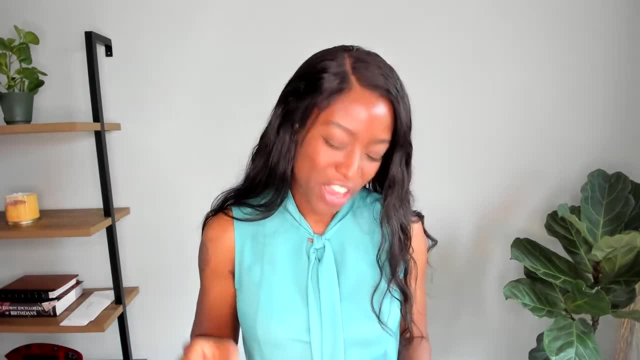 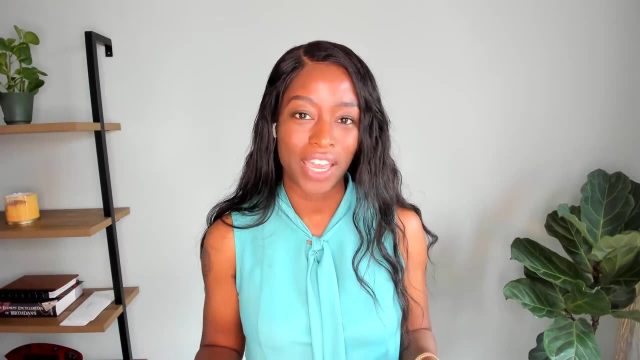 Right, So it works. So just trust me, your kids, they need structure, repetition and lots of heads up. Okay, Again, it is not you, Um, I don't know. some people I think, um, they want to make sure. 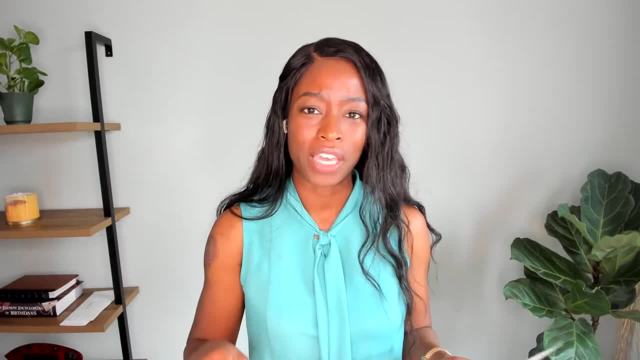 their kids know they have like a sense of authority over them. So it's like that whole thing of do it because I said it Type thing, blah, blah, blah. That's all fine and cool when they get older, But right now, 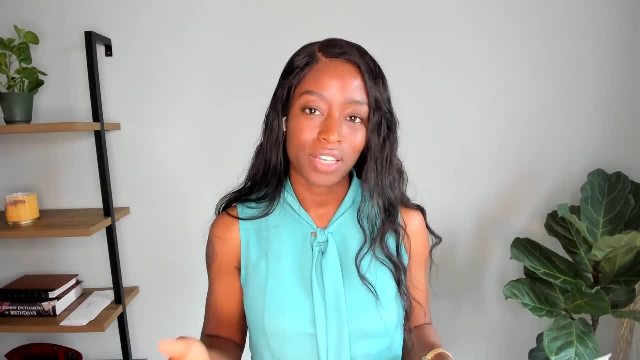 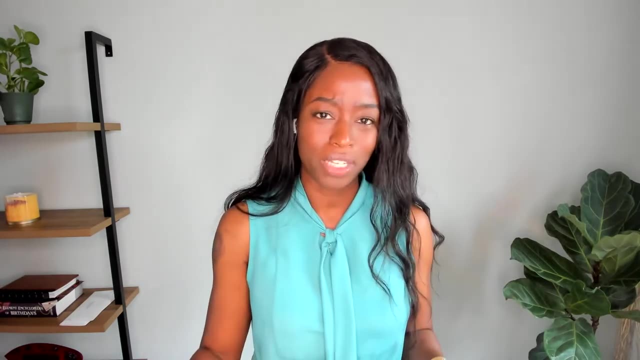 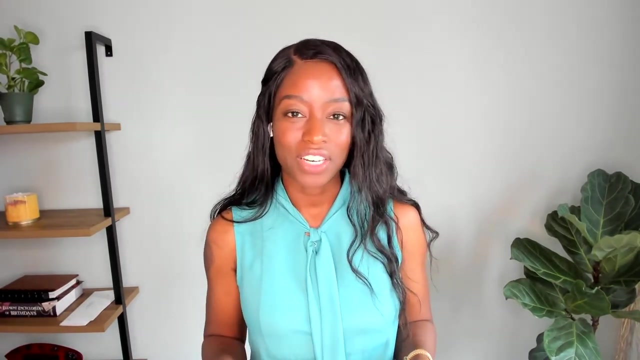 like we're talking zero through six or seven years old. No, guys, give them heads up, pep talk them. They do not like surprises. They do not respond well to that. Okay, You ever seen gremlins? That's what these people are like. So, anyway, let's go on to part two of this video, And these will be the 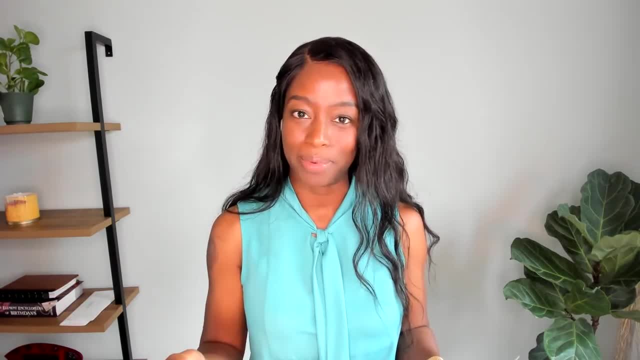 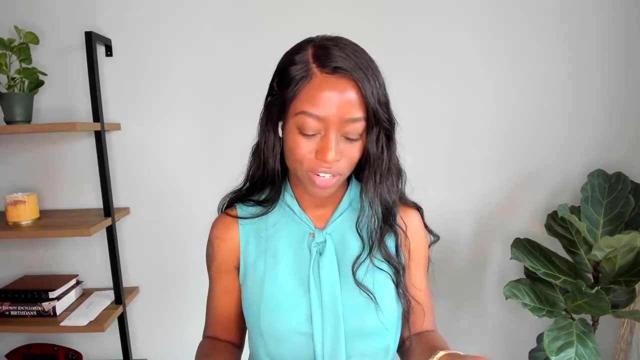 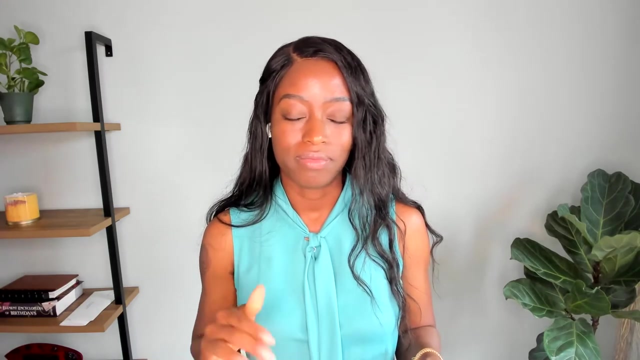 more practical tips that you can start to employ ASAP. Okay, Well, you should do part one ASAP too. um, these are just some easy ones that you can be thinking of as you run throughout your day. So let's talk about laundry Wash, but do not fold. Okay, Don't waste your time, guys. Um, I know that. 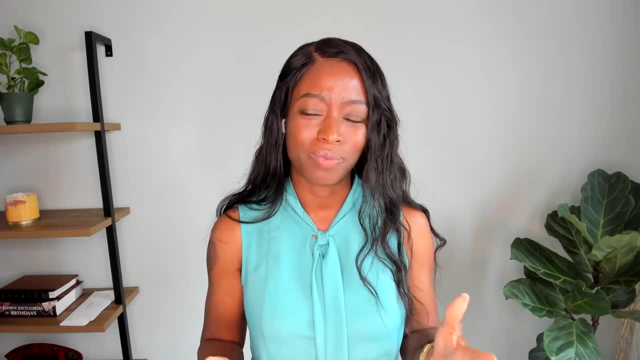 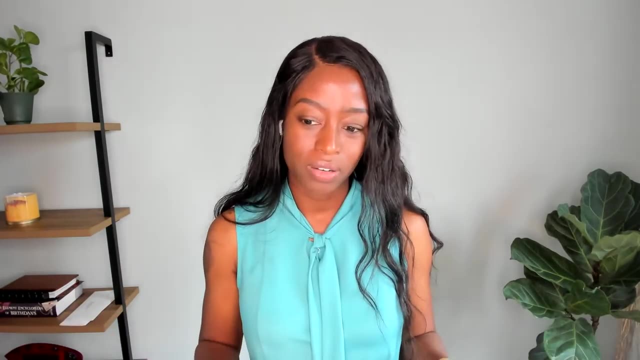 when you have small kids, it seems like they go through like I don't know- three to four times as many outfits as a regular person, for whatever reason. So the wardrobe changes could be warranted. Some are unwarranted. I I don't, even I don't know. I just know that. 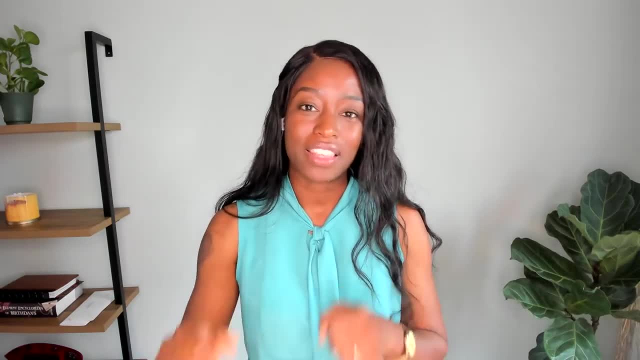 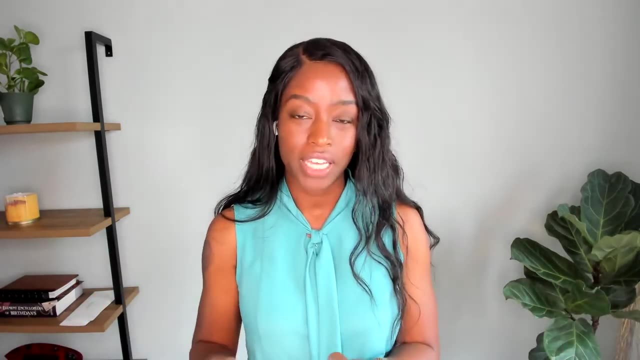 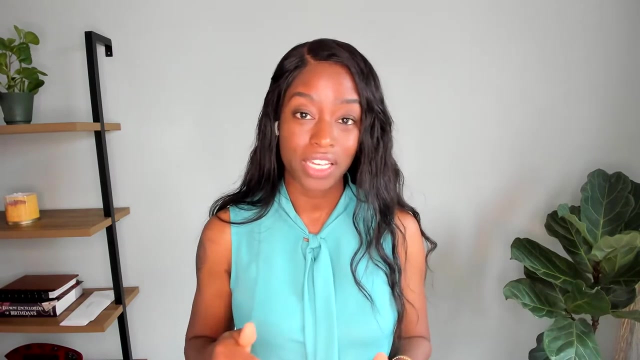 you know, running a load of laundry every single day and then quickly hanging things up has been our saving grace so that things don't pile up. And when I don't do that load a day, you know, like I said, things pile up. Um, we start running out of stuff and that of course creates bottlenecks. 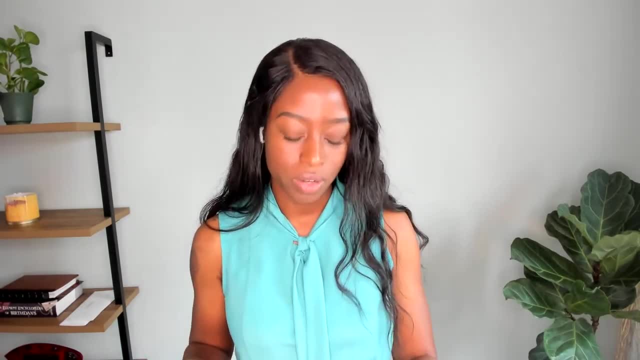 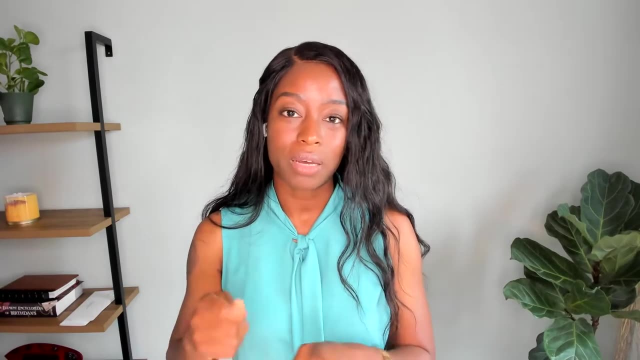 throughout the day that keep us from doing things on time or on schedule or whatnot. So you're definitely going to want to, you know, keep things washed, hang up what you can hang up, fold what you need to, But again, if you're not doing that, you're not going to be able to do that. So I'm 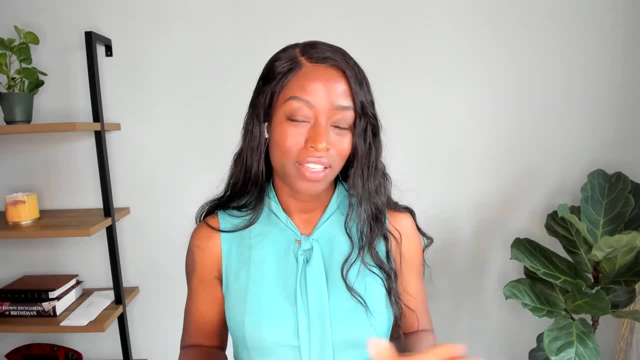 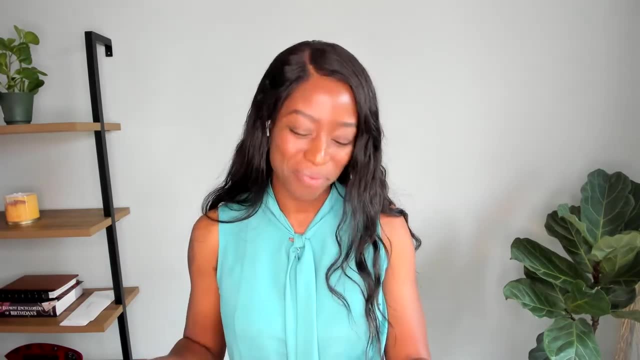 sitting around folding onesies and whatnot. You are the yeah, don't do that. Okay, Don't do that. Um, hang them up, throw them in the drawer. It doesn't matter if they get wrinkled like they're. 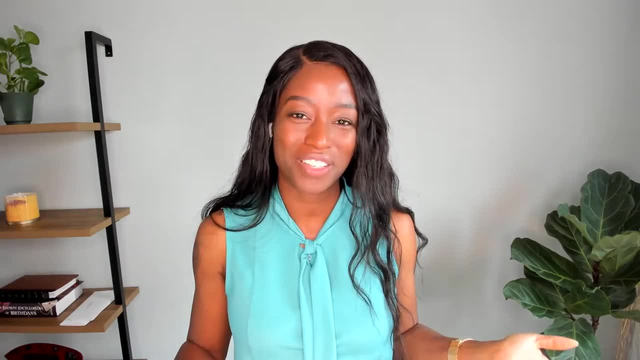 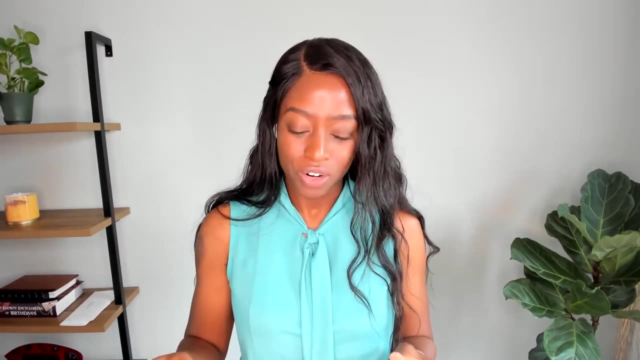 stretchy, you know. So when your kid puts them on, it's going to stretch out and nobody will see the wrinkles. Okay, I promise nobody will see them. Um, while you're doing the laundry, you're going to want to make sure that you're decluttering or getting rid of clothes that are 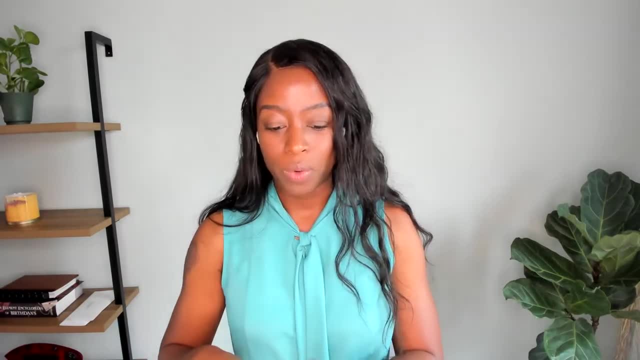 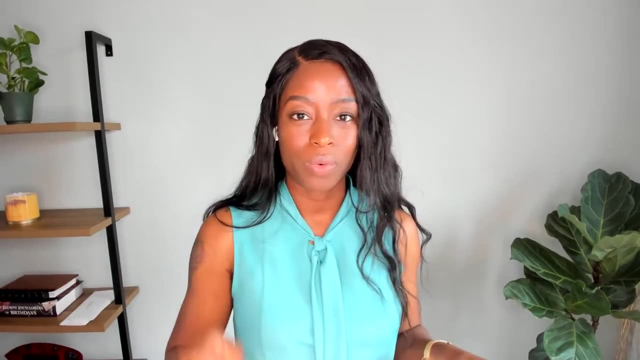 too small or things that look disgusting. So you know, I will, you know, have the clothes and I'll be hanging up whatever I'm hanging up, folding up whatever I'm folding. But there's also a pile where I'm throwing things that I mean we just don't need, right? So it's a bag and I'm just 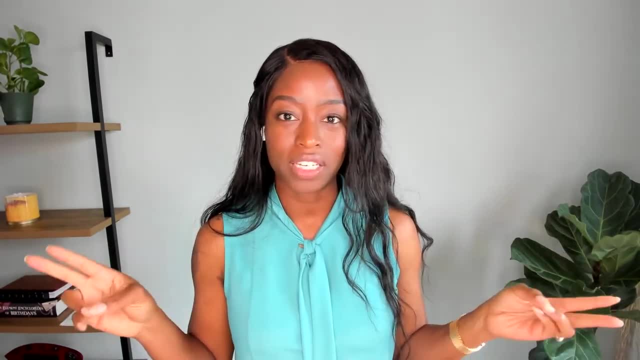 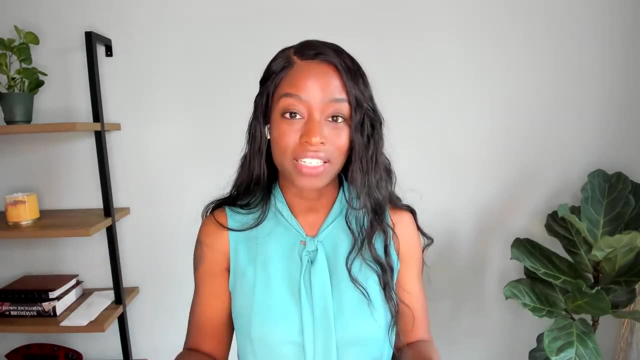 tossing the stuff in there, right there. I don't make like decluttering a big event or um something I have to like plan for or whatever. I just do it as I see things that are no longer appropriate for the kids or myself. 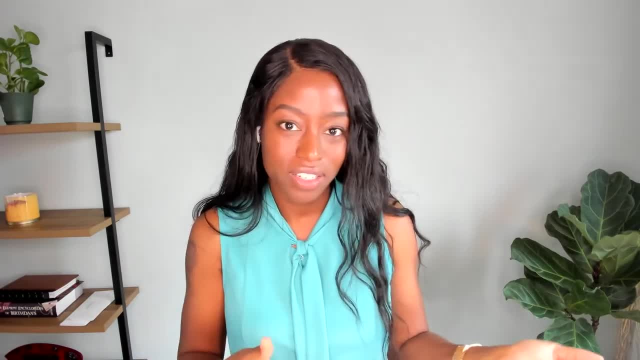 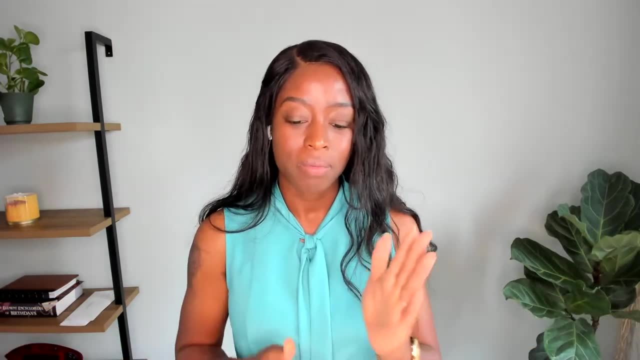 Right. If I see a holy sock or a holy underwear, it just goes into the trash can right then? and there There's. there's no thinking about it, It's just done Right. So you're going to have to kind of be more strategic about doing things you know right here, right now, when you see it. 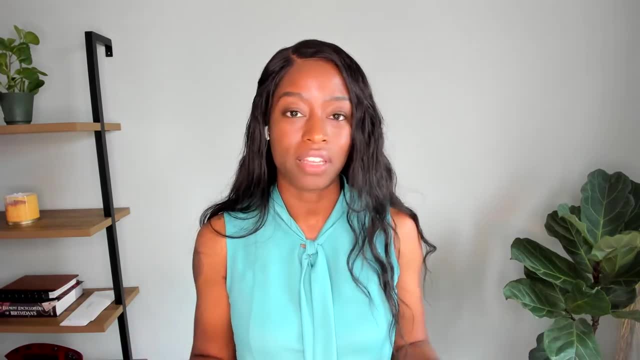 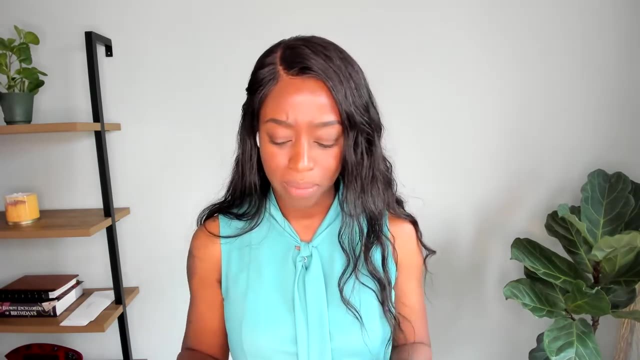 as opposed to: oh okay, I'm going to plan for this later. Like no, it needs to be a lifestyle and approach right: Always getting rid of things that just aren't relevant and don't fit. Anyway, let me get back to that: laundry wash, but do not fold, because 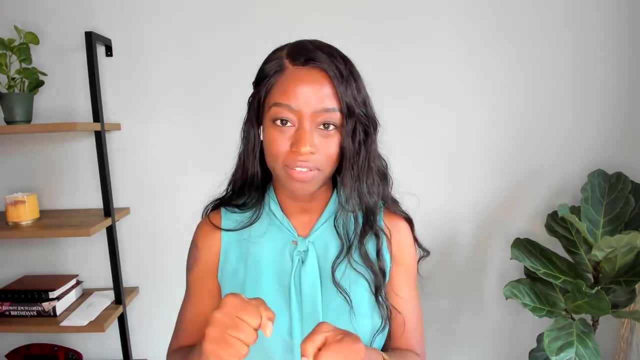 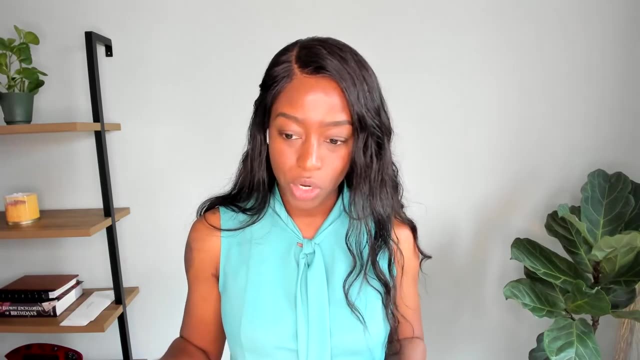 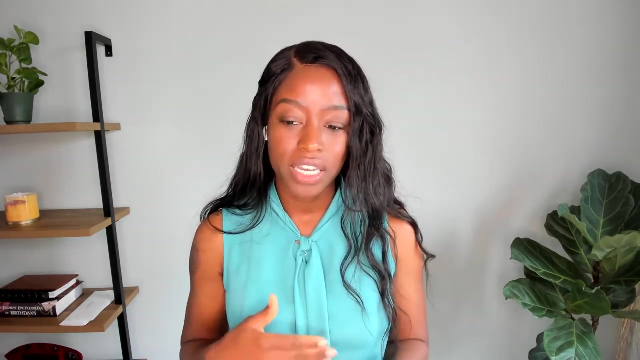 folding takes a long time. Okay, It takes up too much time. Hang up stuff, All right, And keep it moving. Next tip Number two: have fly zones and then no fly zones. So by this I simply mean that if you were someone like me, where I have stayed at home with my kids, basically once they get up, 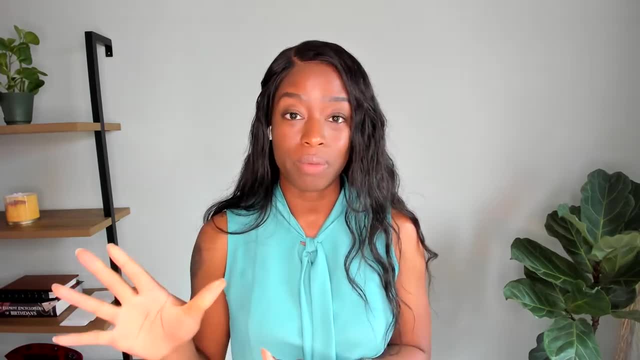 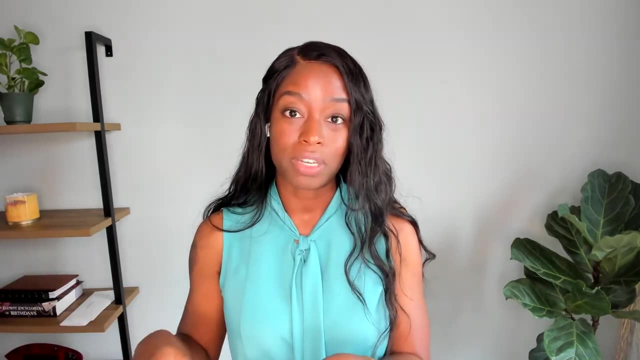 brush your teeth, wash your face, put their clothes on all this stuff. coming downstairs, there is no going back upstairs. I'll go back upstairs to straighten things up or wrap it up, Um, but no, we pretty much spend our day either downstairs. 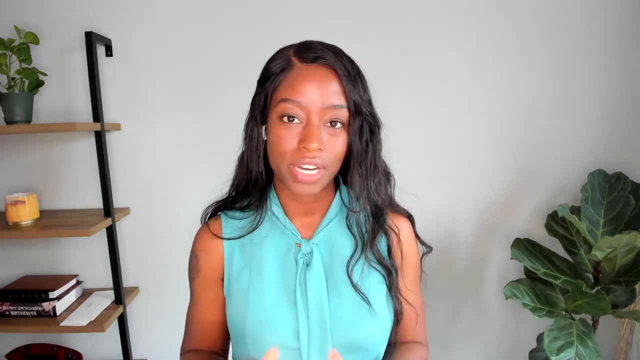 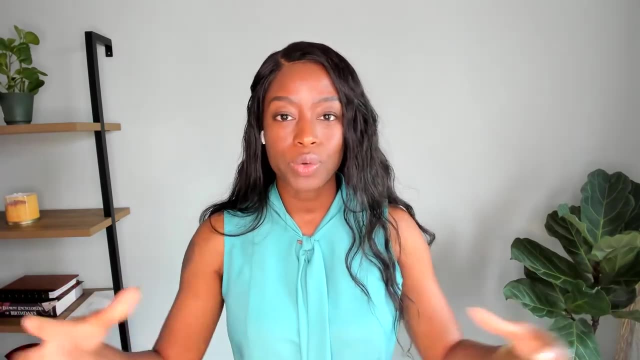 or out and about. There is no running all over the house doing all this craziness. At some point there was, I'm pretty sure, um, in their earlier stages. but the more you can limit their, their reign throughout the house, their reign of terror, the easier it will be for you. 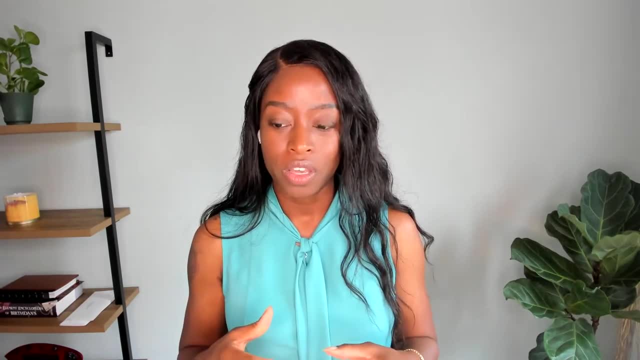 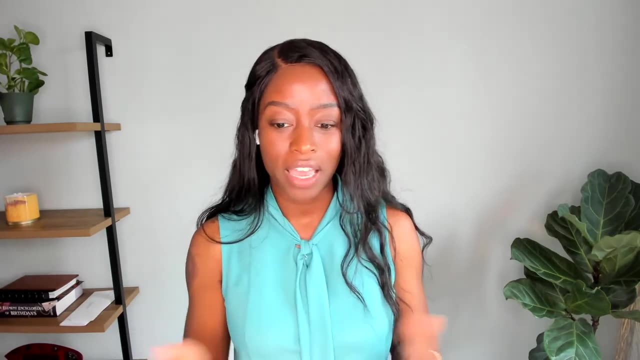 to keep the house clean, All right. So this goes back into that whole. you know, um, you only want to have to do something once. So if I go and make up their beds, I'm not trying to um go back. 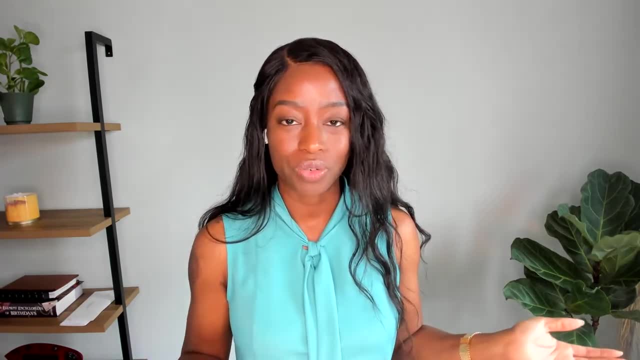 in the room within the next hour. I'm not trying to um. I'm not trying to um, I'm not trying to and see it's been destroyed, Right, That's a bit defeating for me and dis um incentivizing I. 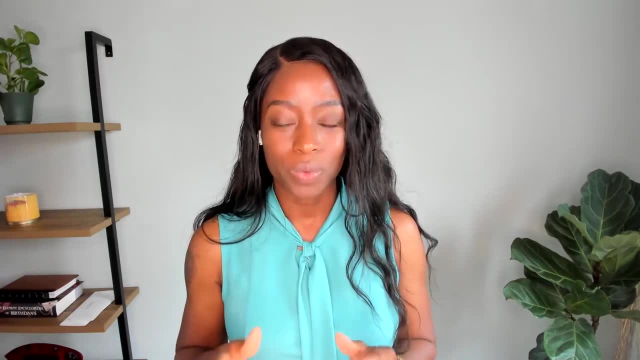 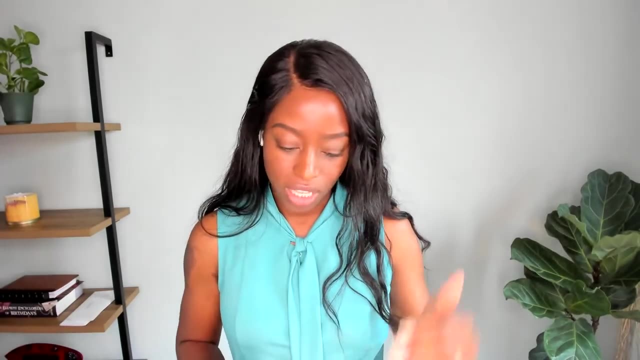 don't even know if that's word. Yeah, I'm just. yeah, Pray for me. So, with that being said, oh, hold on, Let me fix this earbud, Um, with that being said, you want to make sure that they have. 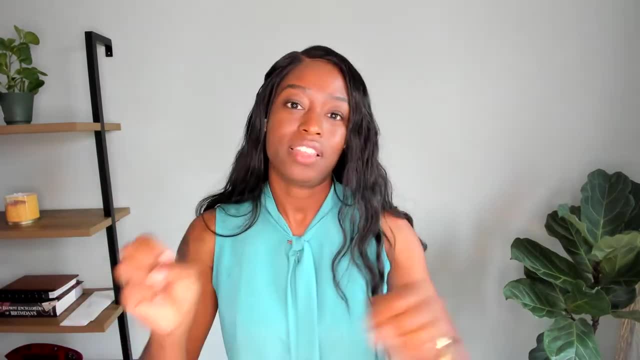 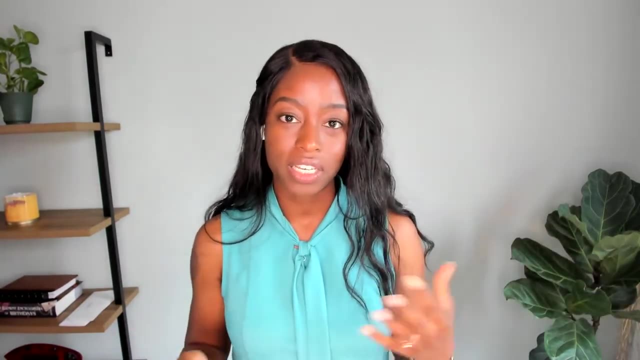 fly zones and no fly zones. Like: Hey, this is where you play, This is where we eat, This is where we sleep. Okay, Again, that structure they also need that They'll respect it. Like, yeah, let me give you some pushback and test. 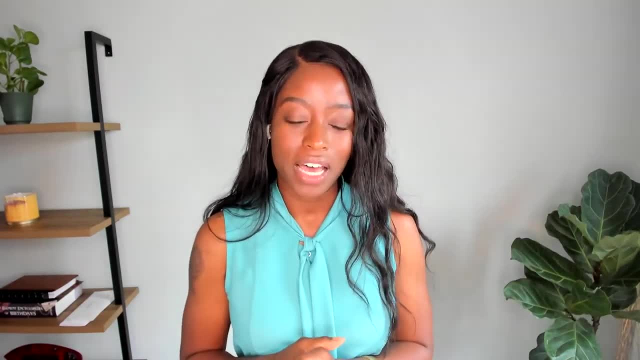 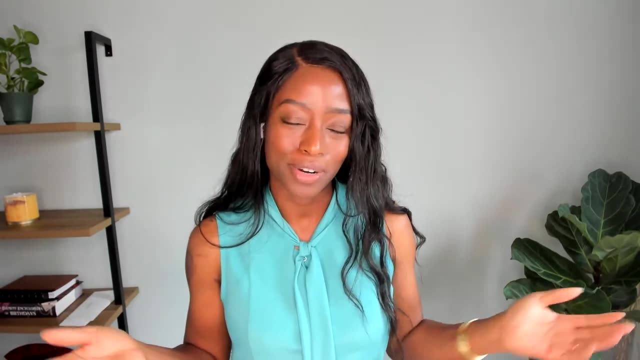 Cause that's what they do, you know, So expect that. but um, they're not trying to be disrespectful, They're just being a human being with, like a, you know, two-year-old brain, baby brain. So, you know, let them know like: Hey, no, this is the area, This is what we do, This is. 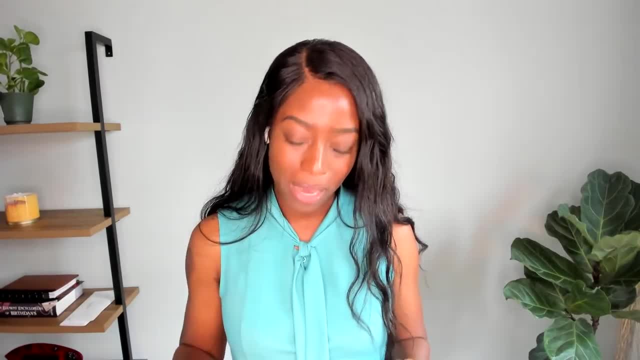 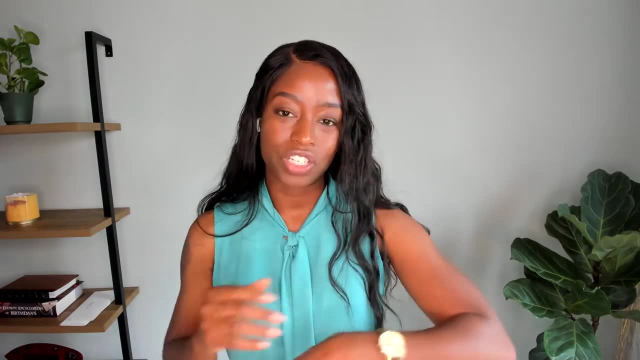 where we do it type thing. Okay, Um, with that being said, think of the jump park. When you take your kids there, you know you have, um you know, access to this park. The other big thing, though, is there's a time limit. There's always a time limit. So, with that being said, you know. 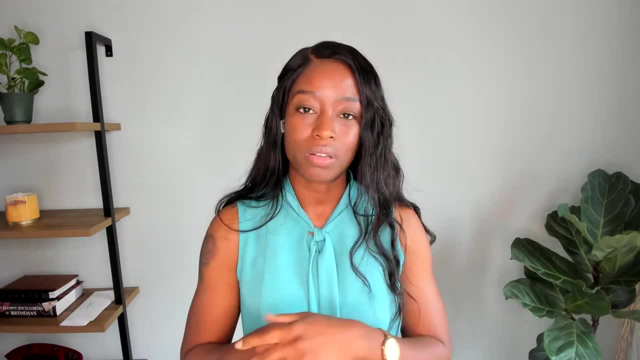 um, it kind of piggybacks off of the whole thing. Give them a heads up right. Always let them know. Hey, in five minutes, you know, we'll be wrapping this up, So if they're in the playroom, 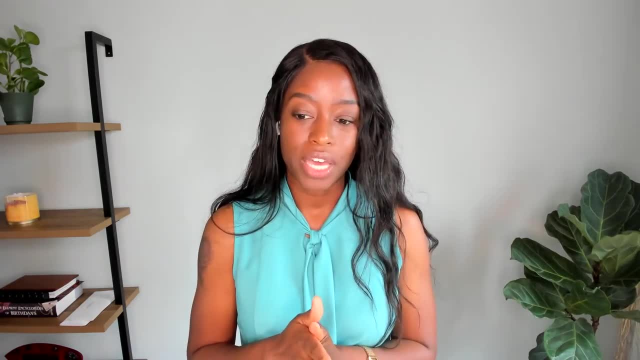 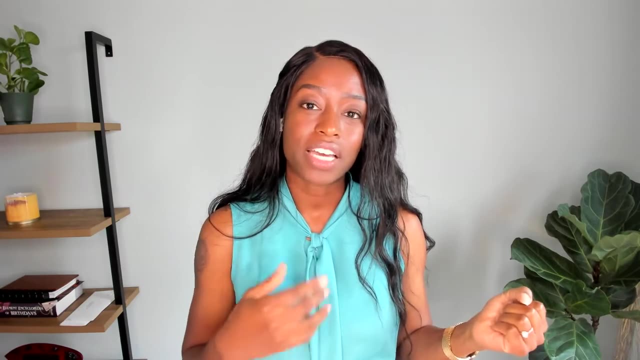 or the play area, and you know that, um, you guys are going to need to be heading somewhere in the next hour. Well, in about 15 minutes, you're going to tell them. Hey guys, in 15 minutes. 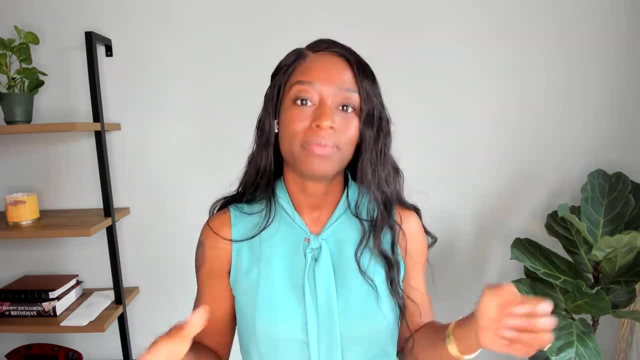 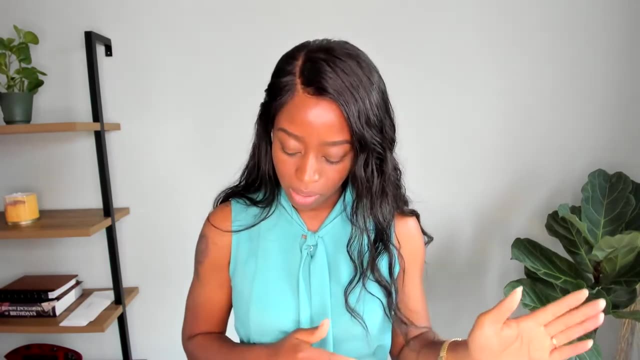 we're going to wrap this up. What does it mean to wrap this up? To clean up? Okay, Together, or whatever. whatever your wrap up process is, but just remember that you need to have fly zones and no fly zones. That's the big piece. Don't let them be all. 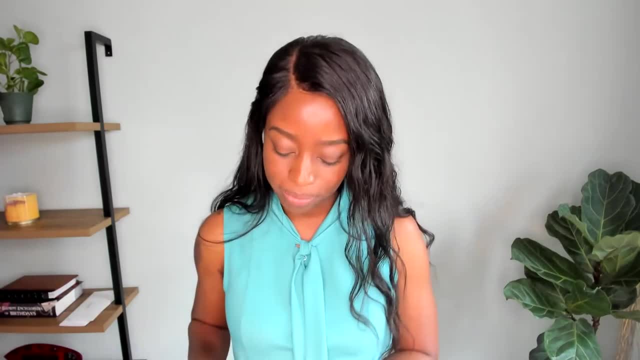 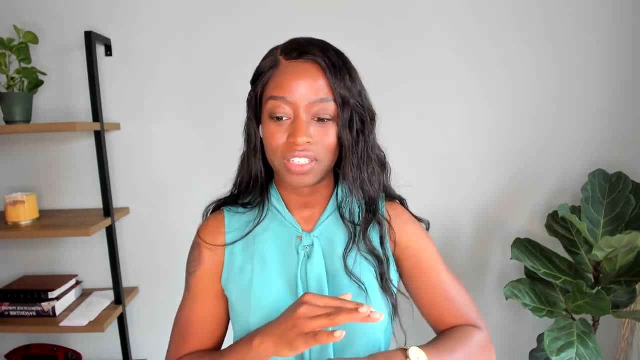 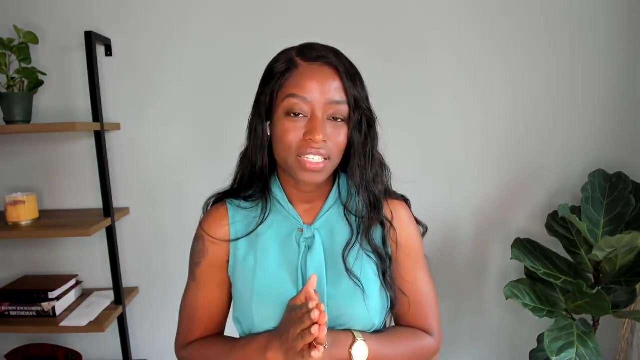 over your house. Don't do it, No, ma'am. Next tip: Stop with all the toys. This is tip number three: Stop with all the just obsessive excessive amounts of toys. I know some people do it because maybe they had a lot of lack growing up So they just want to make sure that their kids have. 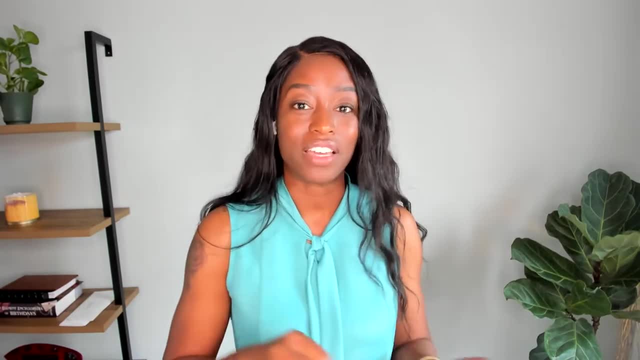 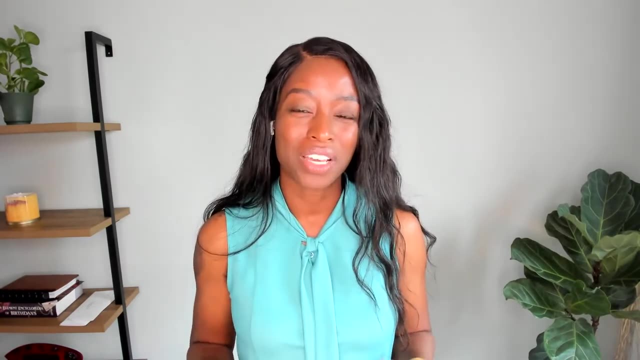 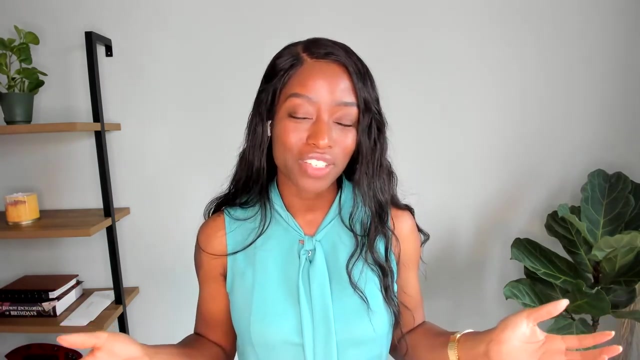 but this is just the wrong way to do it. Okay, Make sure your kids have experiences. Okay, Make sure your kids have, um, you know, nurture and good food. Um, just buying toys just to buy them. And now they're everywhere. The kids are not playing with them. All right, The novelty. 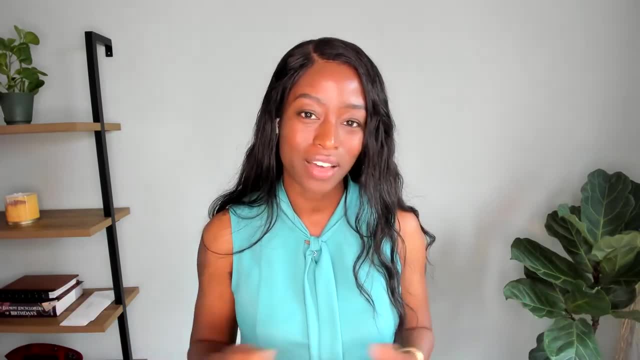 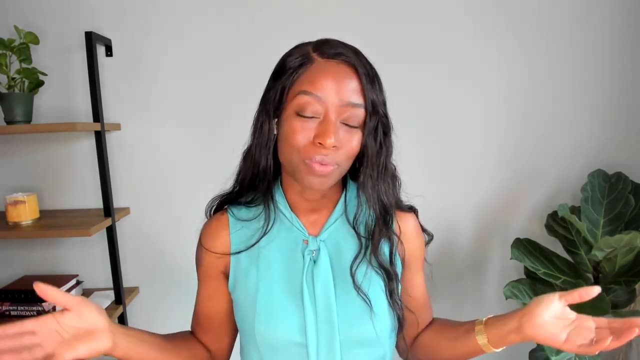 of the whole thing lasted all of a couple hours. And now that toy is broken under your foot, making you mad And for what you know. good job to you. but now what? Pick it up, put it in the trash. Um. 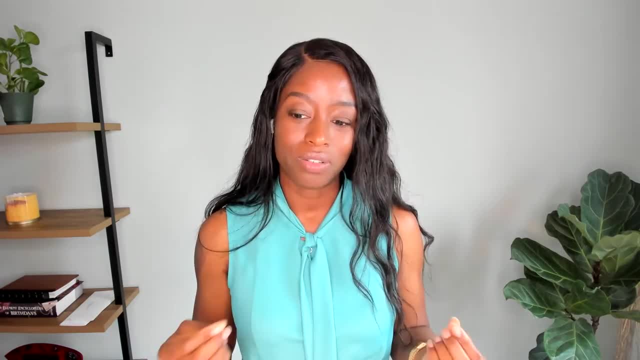 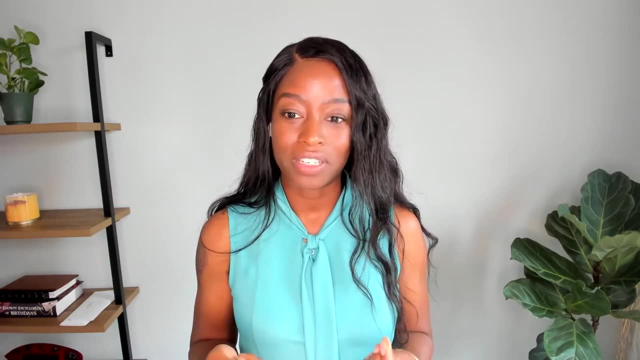 yeah, If you are, um, unable to say no to your children, that's something that you're going to have to work on, because, again, as a parent, your job isn't just to say yes to everything. Your job is to teach them, you know bigger lessons that will help them be a well-rounded 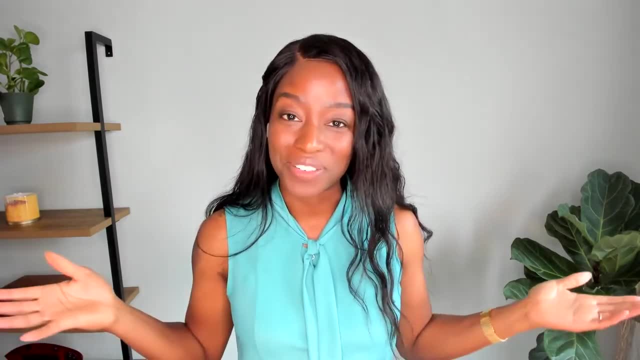 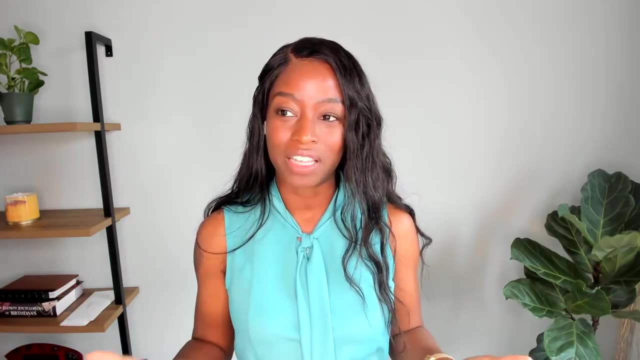 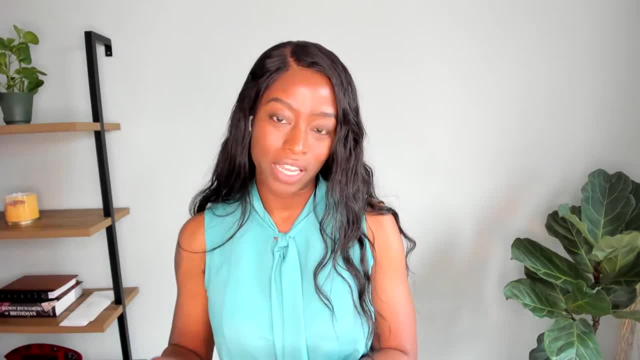 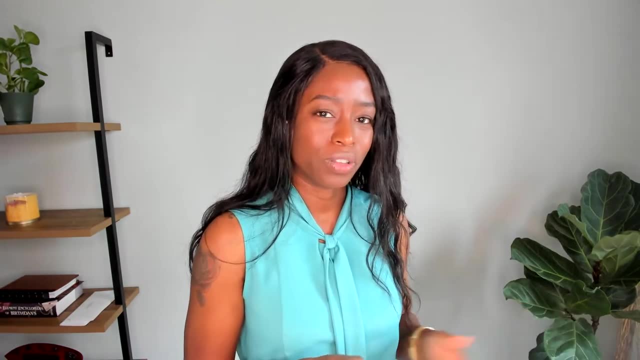 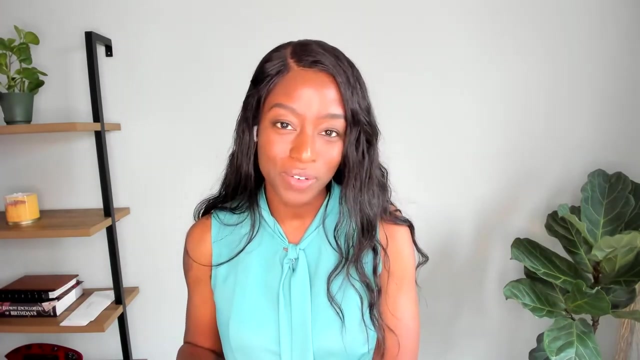 the number of toys or parents were or were not able to buy them impacted that Okay. So it's not like the more toys you give them, the more successful or the more, the more loved shall we say. they know they are right. Your kids will know they're loved when you put your phone. 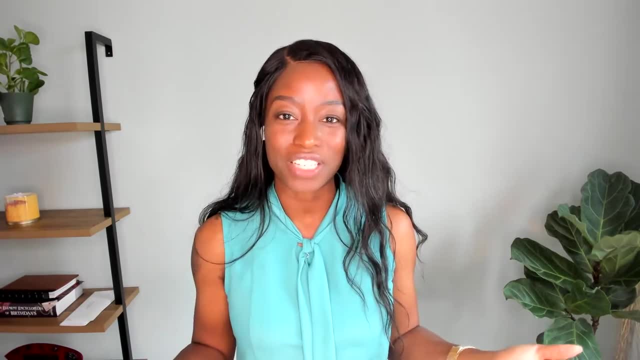 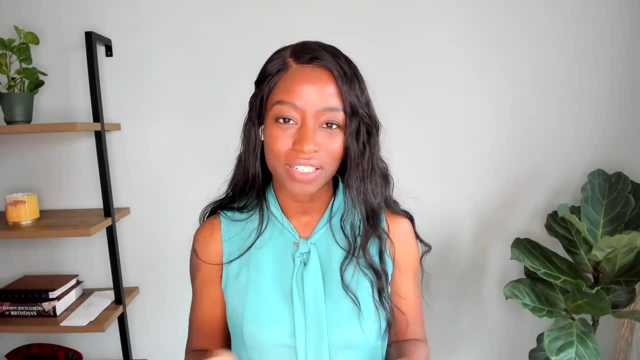 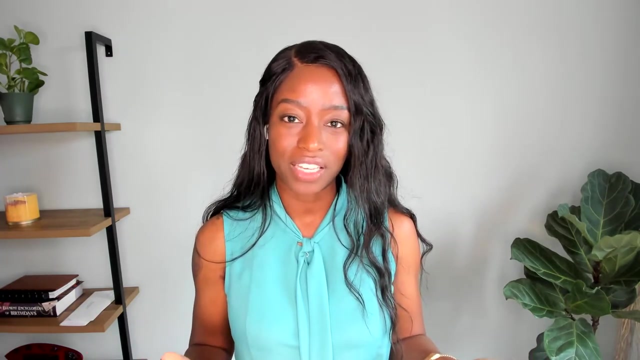 down and you actually make eye contact with them and have a conversation right, Or when you sit down with them and draw a picture with them. okay, experiences, guys, um, you can also make sure that they learn um the art of decluttering right and getting rid of things that we no longer need. 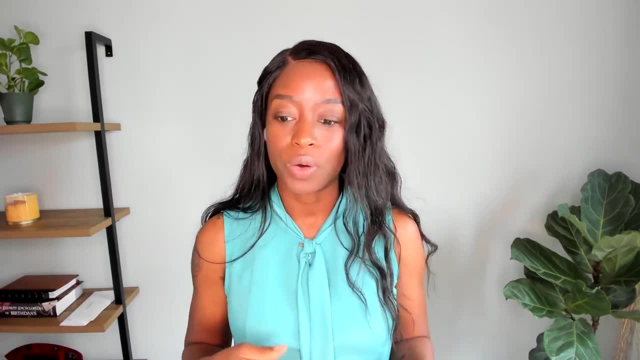 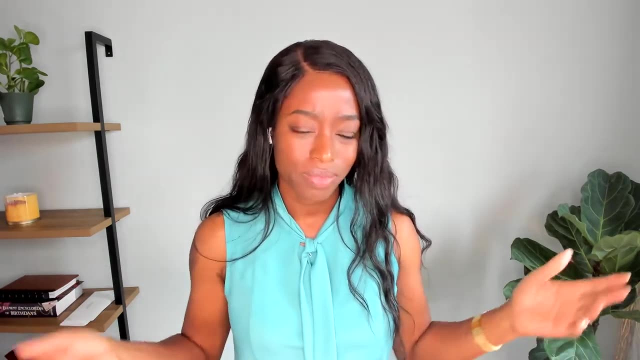 so that they don't have attachment issues to things as well. so before we go out for christmas, of course, that's when we gather up all the toys we don't want or are broken and we put them in the trash. if they're in good condition, sure you can give them to goodwill or whoever. let me rewind. 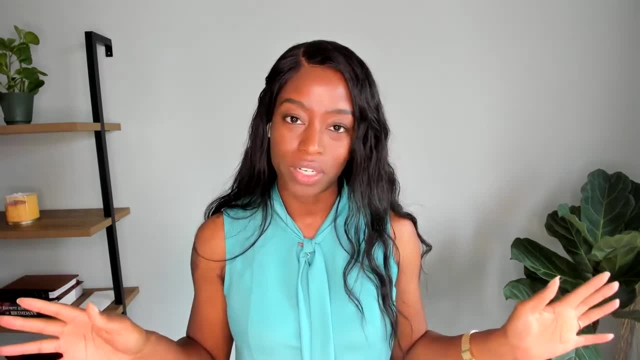 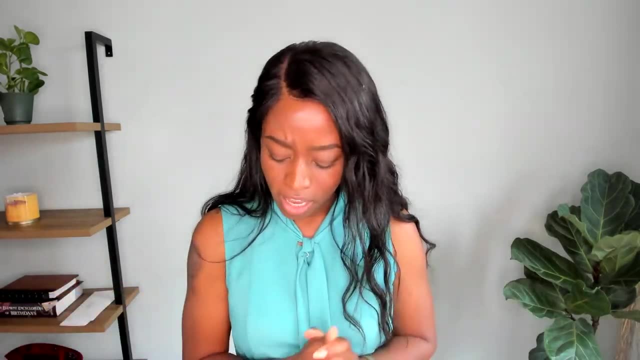 yes, i'm always putting things in the trash, right, not everything needs to go to the goodwill. some of you guys are giving people literal crap like: don't do that, guys put it in the trash. okay, yeah, i'm just saying all right, so let's go on to the next tip. tip number four: have baskets with 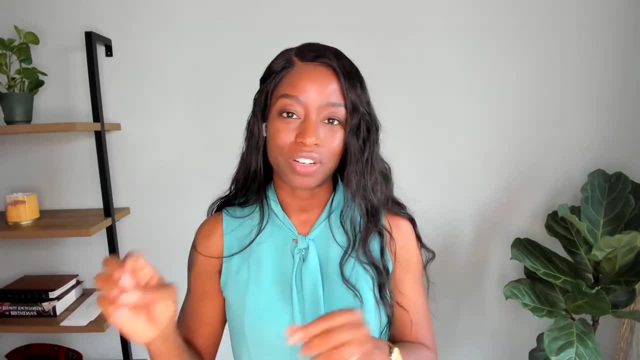 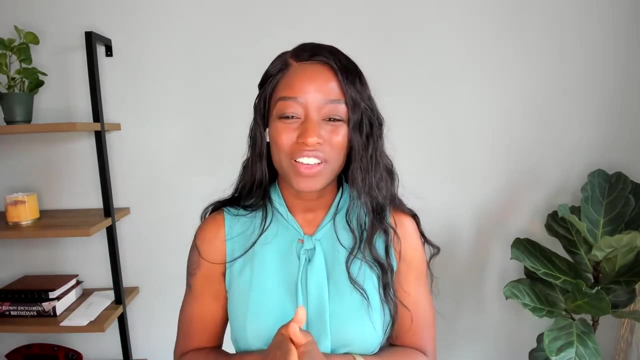 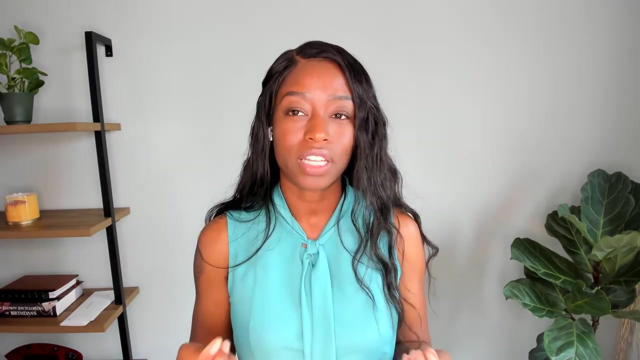 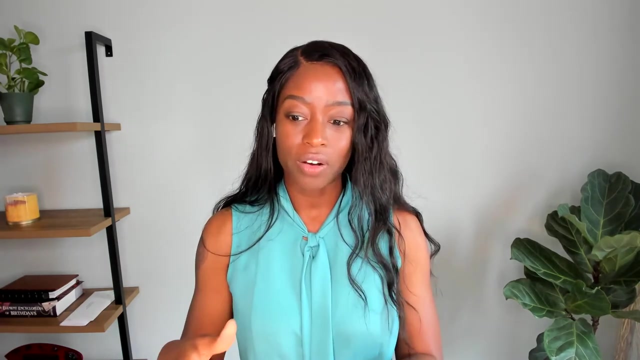 clear labels, have totes that are clear and with labels and do not put lids on things. so kids, when they're that young, and even some adults, right, this really ties more so into your clutter or organization personality, right, so i'll use myself um there once upon a time when i 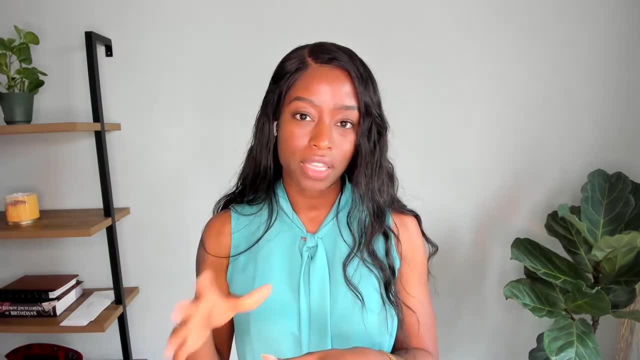 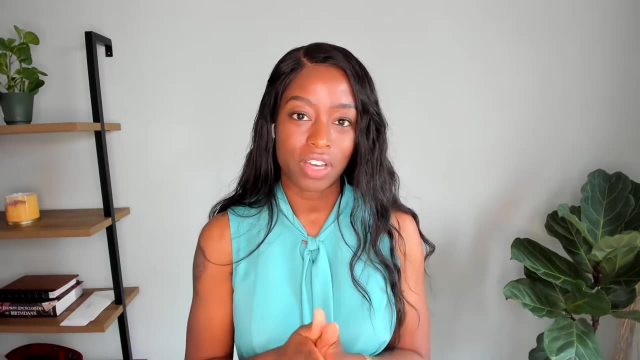 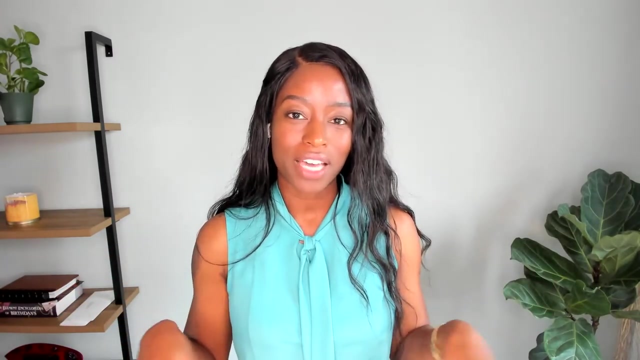 was living with my parents. they had a laundry hamper in the laundry room and it had a lid on top right, and so i like to keep things clean. you know i can be very particular about my space, but i realized that everyone was putting their clothes on top of the basket and around the basket. 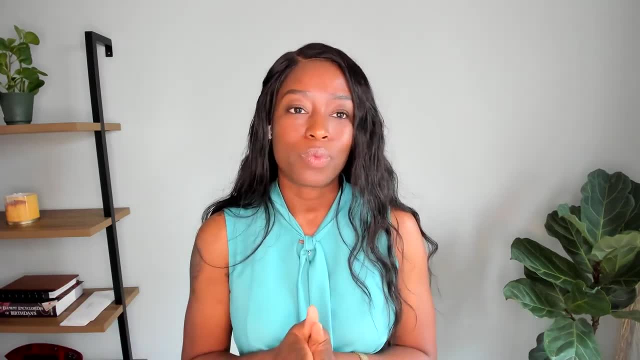 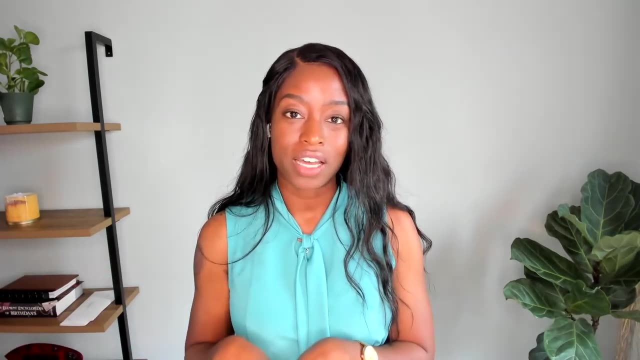 including myself. so i'm going to show you how to do that. so i'm going to show you how to do that, right, and i'm just like what in the world? and then one day i realized, okay, let me just take this lid off, let me hide it. and all of a sudden, now the clothes are inside the hamper. oh genius. 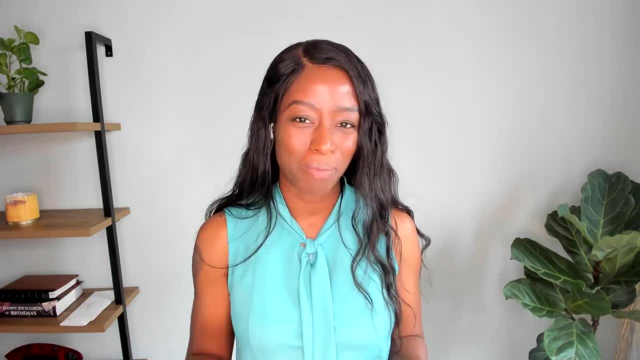 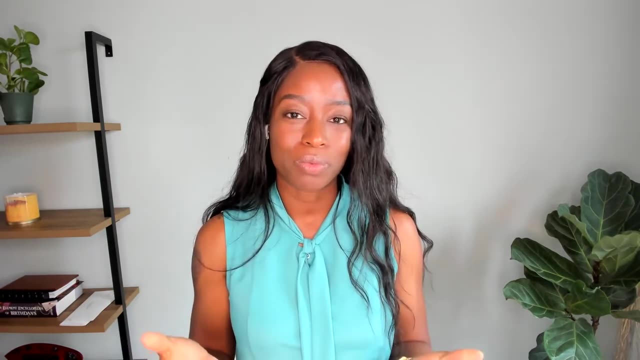 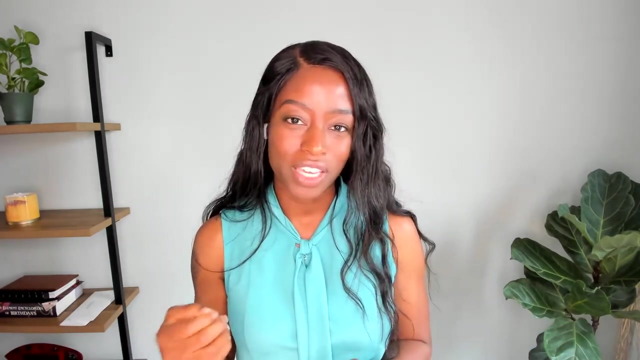 right. so that little thing, it was an obstacle, it was a barrier, and that one little tweak though, um, or that one barrier kept the room, the laundry room, and an absolute mess, and removing that barrier completely changed the situation. so, with that being said, with your kids, with yourself, whatever you may notice going on, even with you, right in your own, your own spaces. 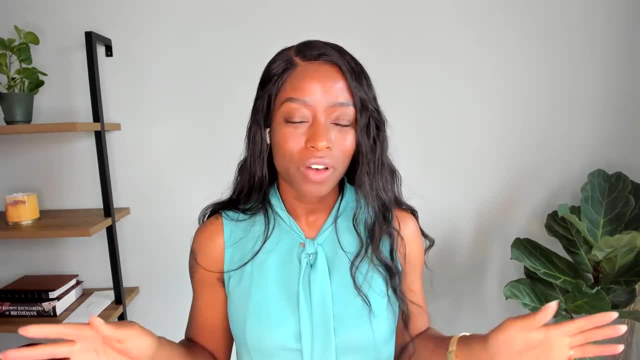 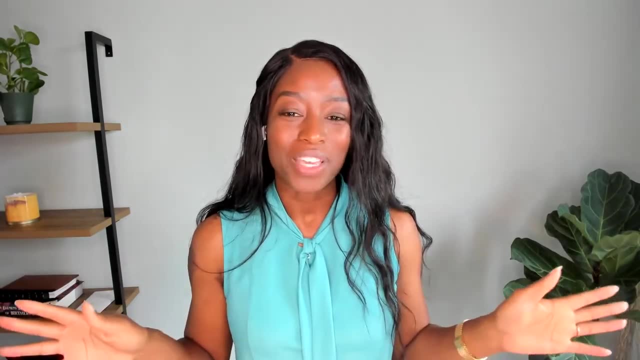 or how you operate. there may be barriers. that don't call it lazy. yes, it can seem lazy to not want to take the lid off, but we're just humans, guys. okay, like i'm a human, you're a human. we can't judge each other. we all have our quirks and it just is what it is. so take the lids off. um to make. 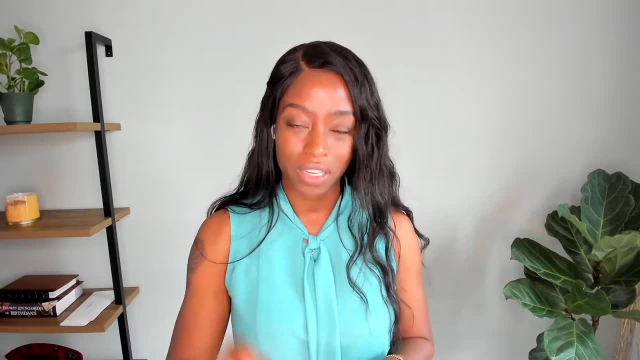 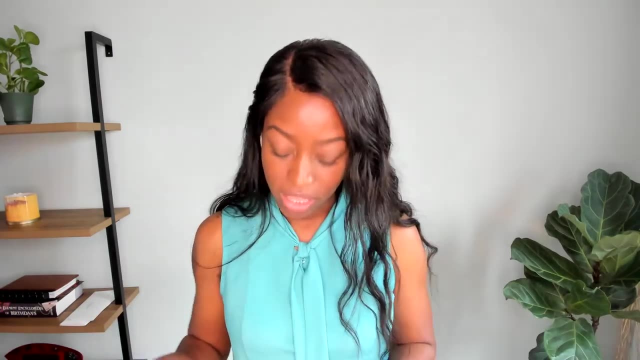 putting things away a lot easier, okay, and this is especially if you notice that things are piling up around containers that you may already have in place. so i'm going to show you how to do that. okay, so i'm going to show you how to do that. so i'm going to show you how to do that. 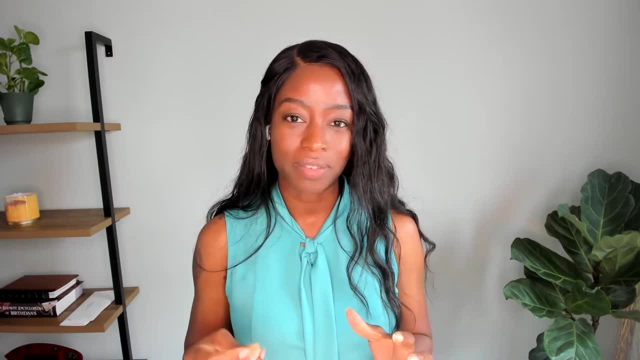 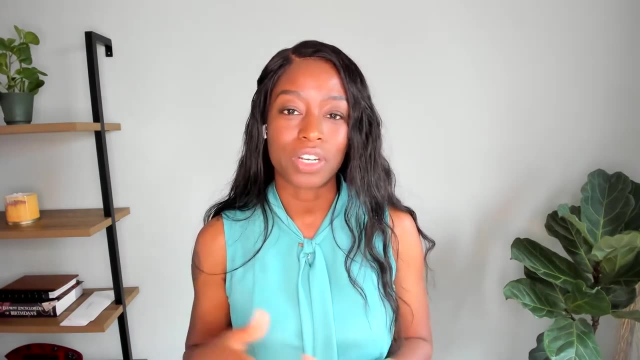 the labels, on the other hand, definitely help with the kids because it they like to know that they're doing something right. right, your kids are in an age where they want to do things. they want to do what they see you doing. you know, if this uh basket says, 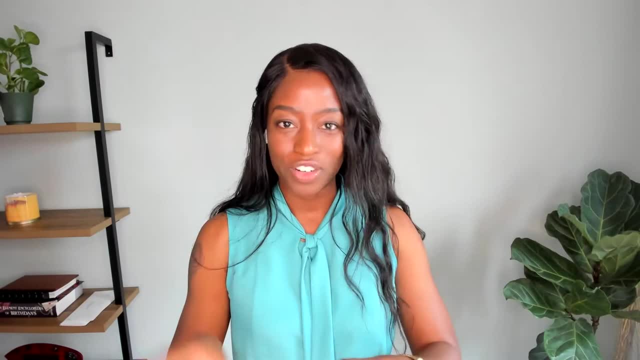 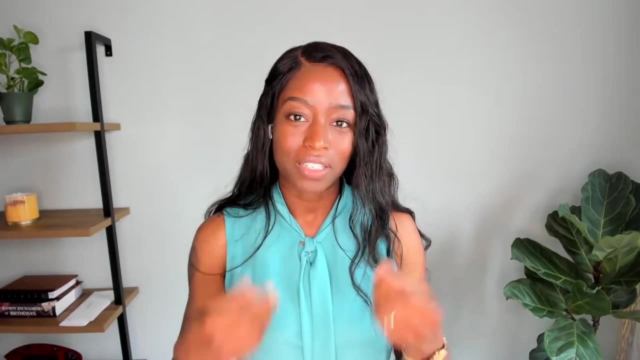 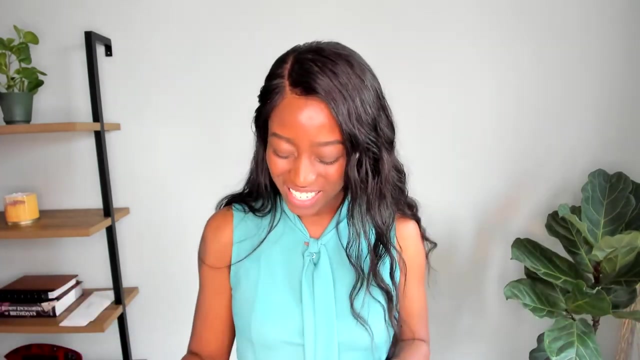 green things go in here. they want to know that they're putting the green things in the green basket. so those labels are kind of like a reward for them and it engages them because it's something for them to learn, something for them to remember, and it just works. okay, it just works. so, yeah, have baskets with labels and have clear containers with. 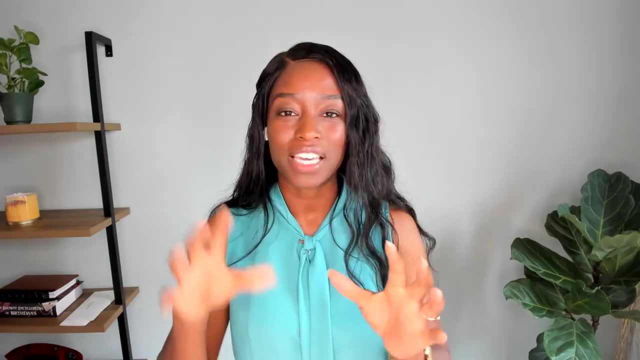 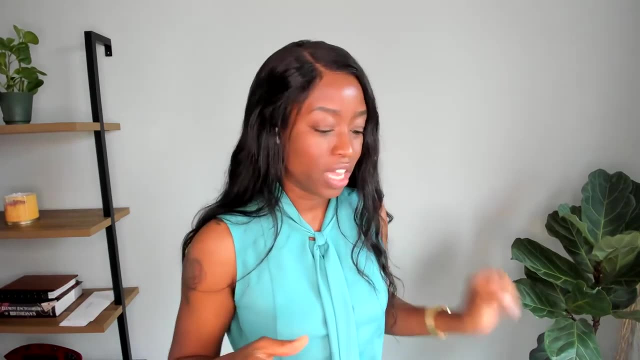 labels. oh, the clear container part is just because a lot of times kids want to see their stuff right, they're visual, so it's like um, it's kind of like if: if i put things away into a drawer a lot of times, i won't remember that i put it there right, so i'm going to forget all about it, even though. 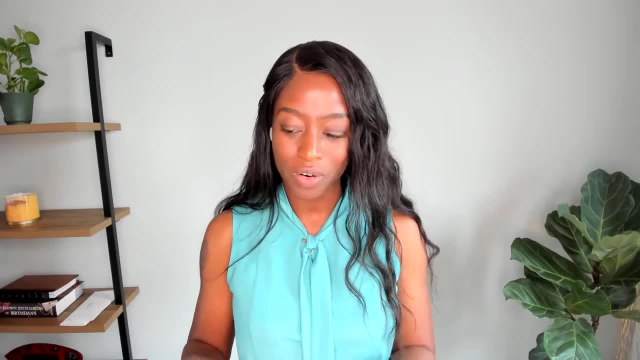 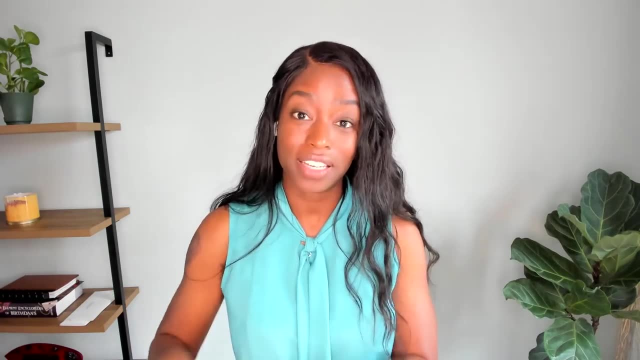 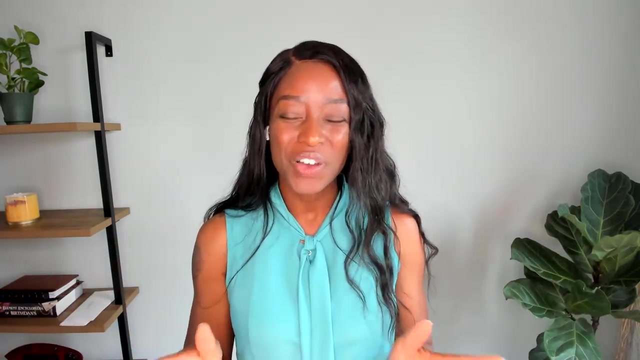 it's super important. so i put things that i want to use, whether it be jewelry or a specific ink pen or whatever it may be. i leave it, like on my desk or somewhere where i can see it, because if i don't see it, it doesn't exist. and again, i don't know why. i'm just don't know. um, ask god. so, with that being, 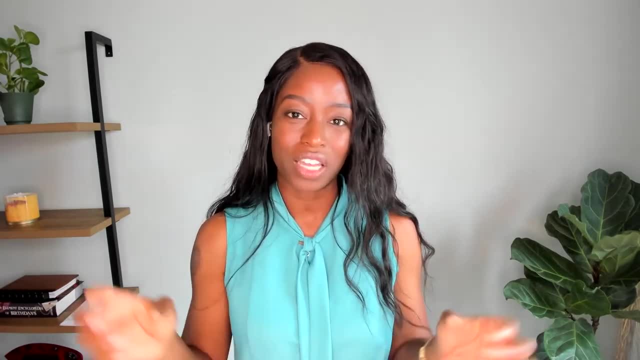 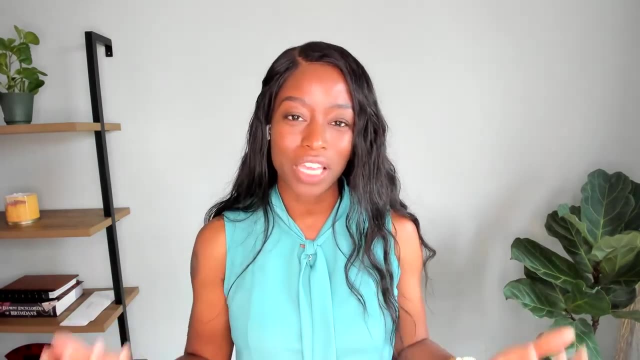 said, though, kids that's kind of like, uh, one of their quirks too: they like to see their stuff. so you want to make sure things are organized and able to be put away. but, again, clear containers definitely helps, you know. keep them on board with the whole thing and not having panic attacks. 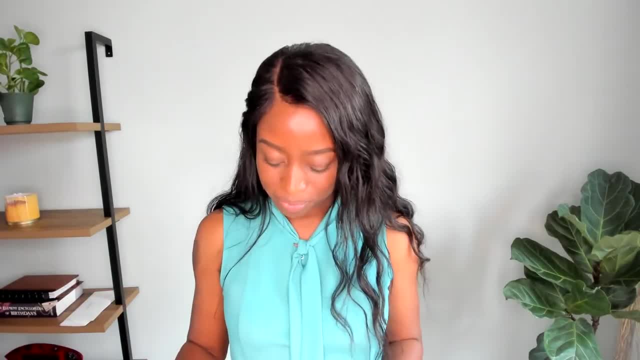 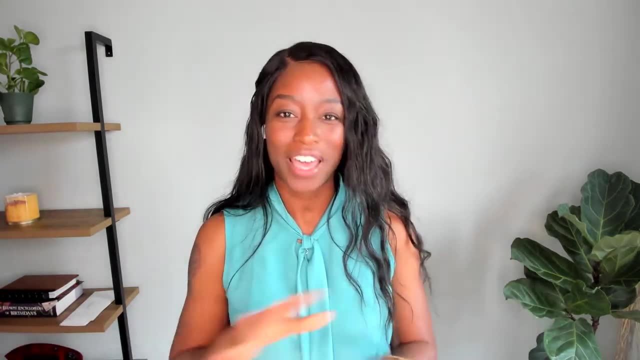 because they can't see batman anymore. you know, you get it. yeah, all right. and so the next tip, number five: all right, there must be a beginning and an end to everything. so what does that mean? well, let's look at it this way: there's a beginning to the day and 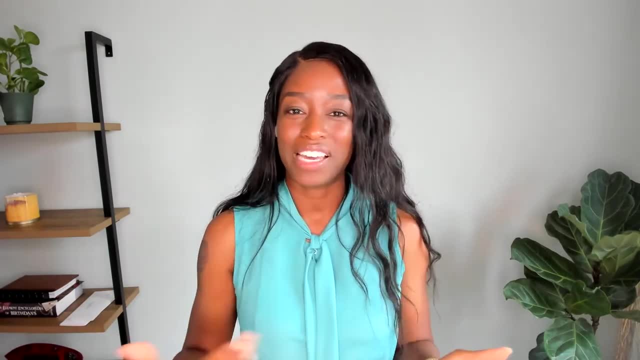 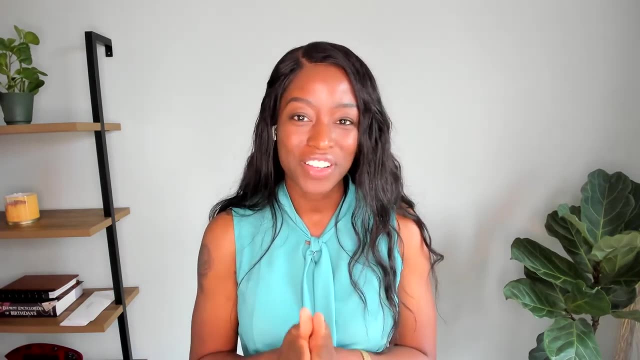 an end to the day, and i know that for some of you, like your kids may not have a bedtime or you know there's not a time- your house actually shuts down and that is wreaking havoc on your life. okay, there has to be an end time to the day where the chaos stops. 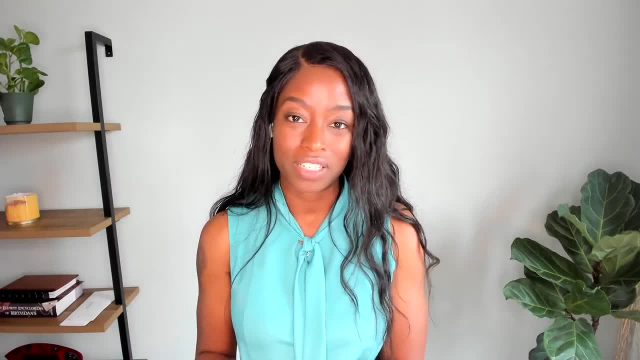 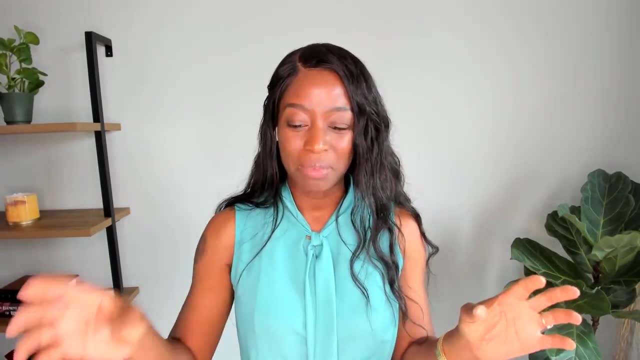 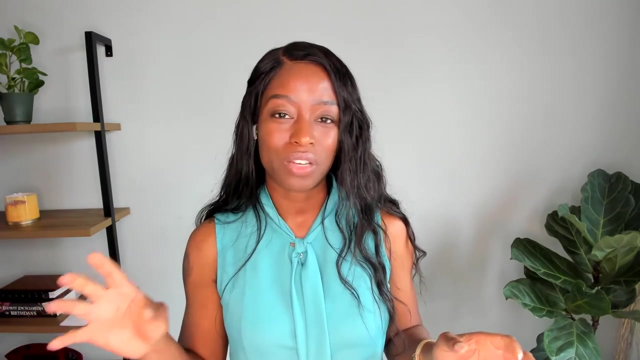 absolutely stops. so number one: there needs to be a beginning and an end to your kids day. there has to be a beginning and an end to your day and that needs to be marked with very specific routines. you know what does the beginning routine look like for the day? what does the end routine for your kids? 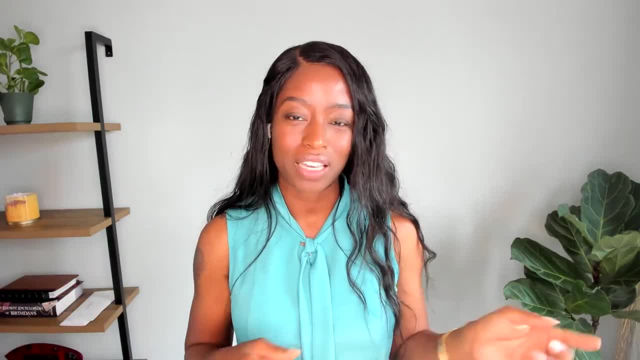 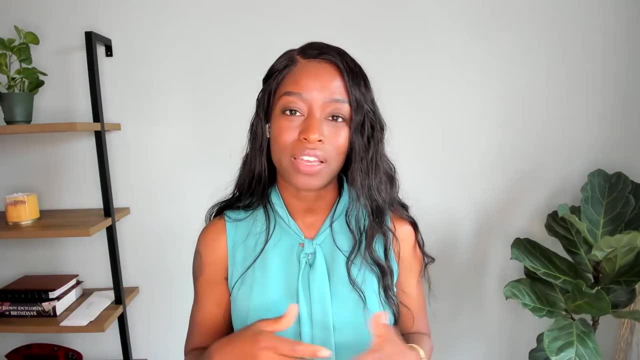 look like you know at the end of the day- so it could be- they come home, they take a bath, they eat dinner, uh, brush their teeth. you guys watch whatever together or you talk or whatever it is that you do, and then you guys go upstairs and you guys go home and you guys go to bed and you guys go to bed and. 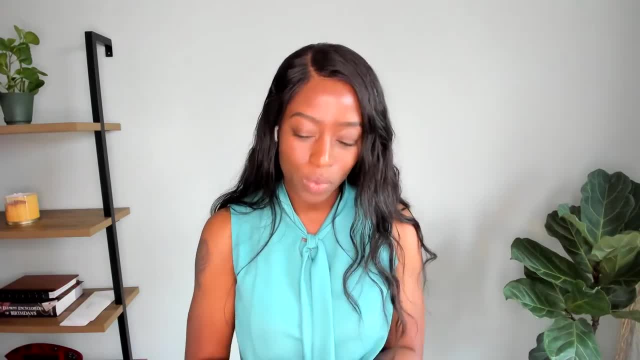 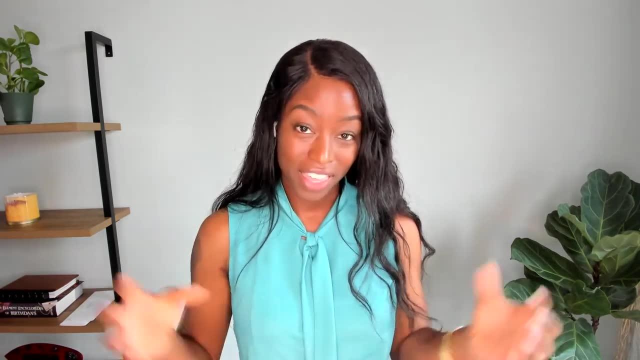 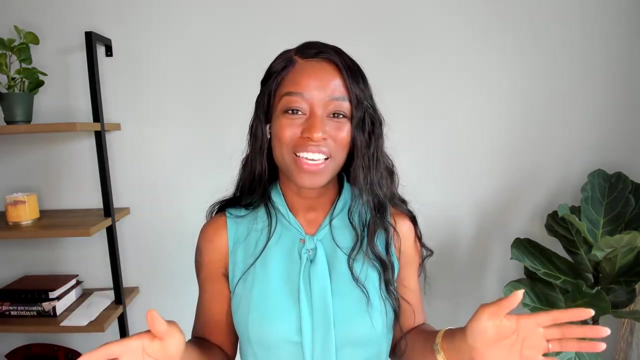 you guys go upstairs, read a book, go to bed. boom, that's the routine. whatever it is, you know, let that be the thing, because again, it helps to enforce that structure, that repetition. but then this is where your time to actually do things, or to even think, comes from. okay, because for me i know that. 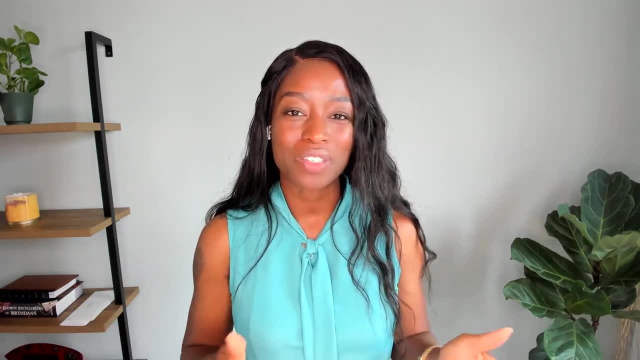 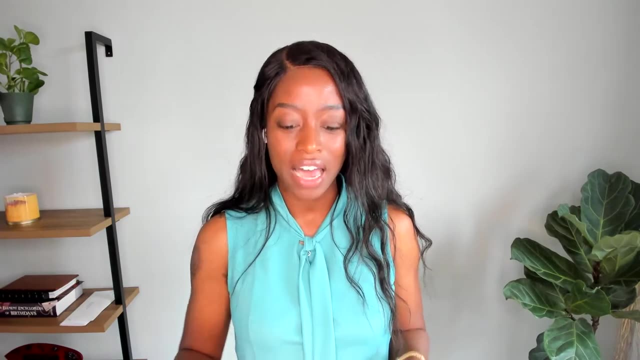 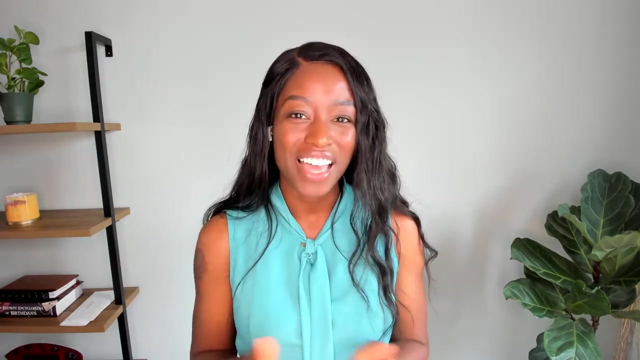 you know, my days were literally filled with chaos, but i knew it was going to come to an end like, okay, yeah, i was only glad to make it three more hours, that's it right. but imagine if i did not have like a very strict cut off time. i mean, yeah, i would not be here talking to you, i would not. i 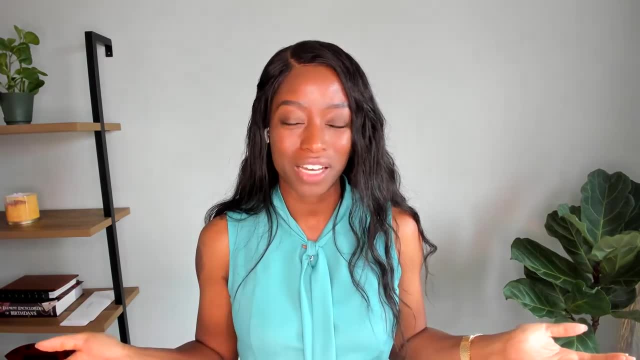 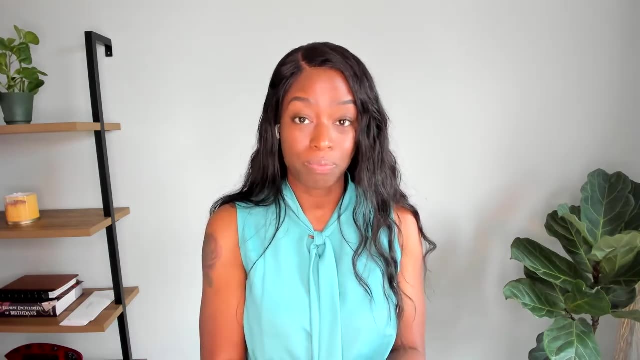 would be in the bed somewhere, still just trying to recuperate from, you know, the past few years. so there has to be a beginning and an end, the same with any activity throughout the day, right? so breakfast, there has to be a beginning and an end, otherwise you will cook breakfast and your kids 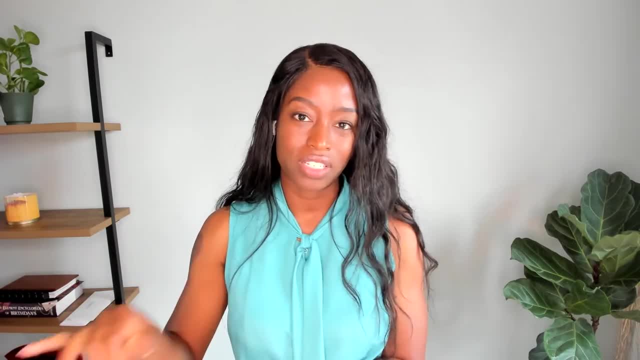 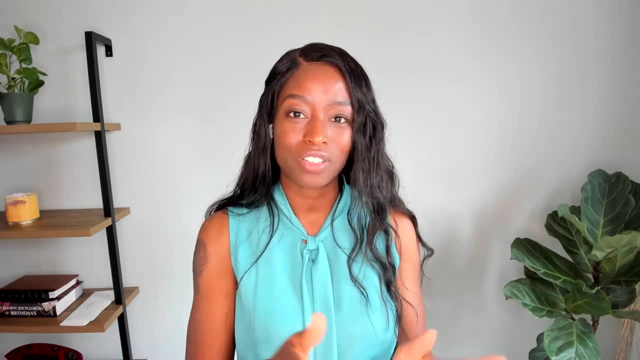 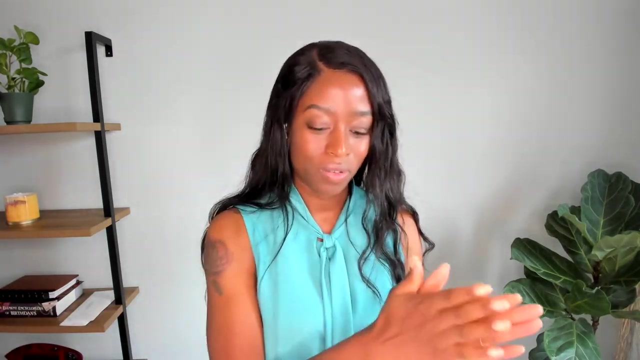 will have you in the kitchen from breakfast, through lunch, onto dinner and through to midnight, like taco bell. this is not taco bell, like no. there has to be a beginning and an end there's. we're doing this 20 minutes and wrap it up and we move on to our next activity, whatever that is. so your day should be a. 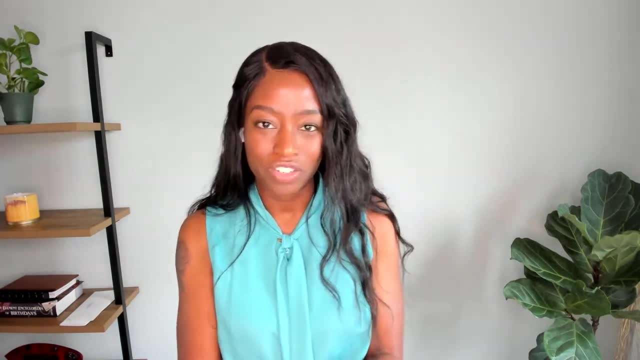 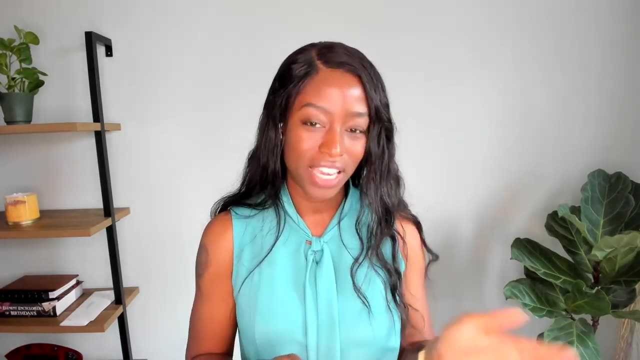 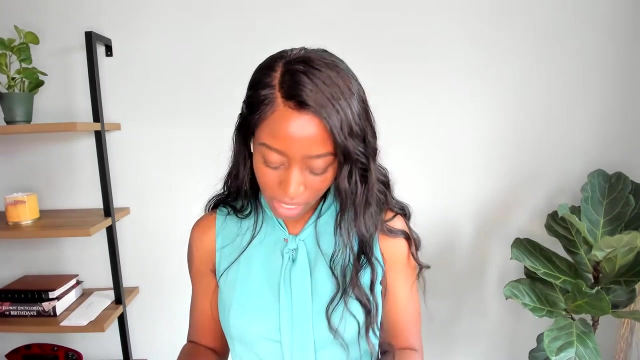 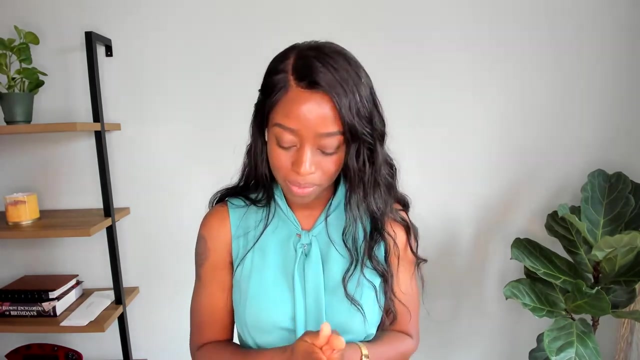 series of, you know, activities, wrap-ups and transition to the next thing. okay, but there's a beginning and an end with everything. we go to the playground beginning what time does it end, i don't know. wear them out, though. wear them out, yeah, make sure i don't miss anything. all right, so let's move on to the next tip, which is: yeah. 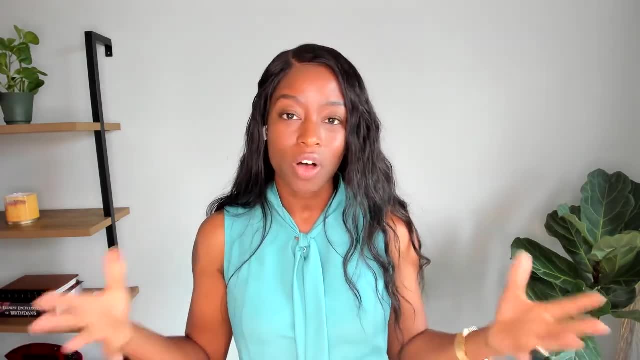 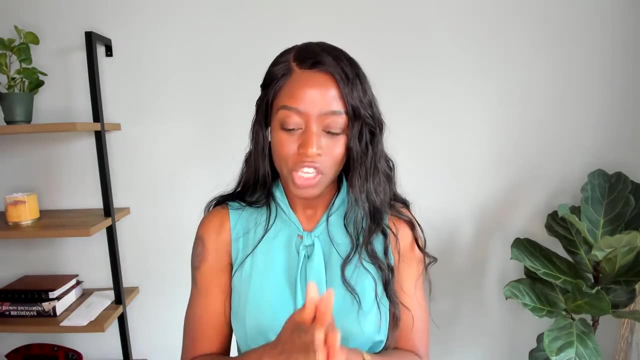 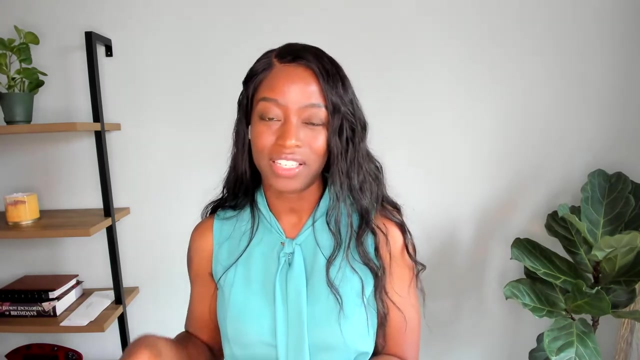 number six: you should not be cleaning all day long. okay, that like don't do that. that's just a very depressing way to live. you need to sit down, you need to plan out your day. okay, and again, the previous tips kind of feed into this one. there should be: imagine if you hired someone to 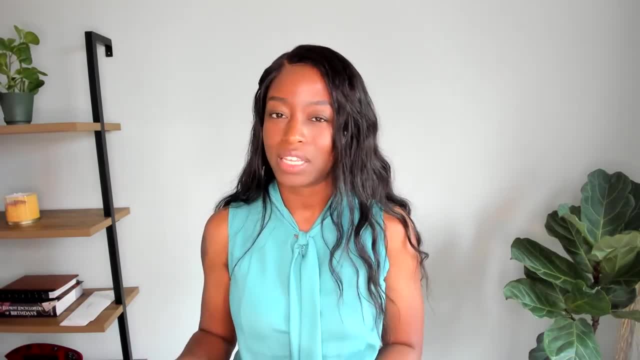 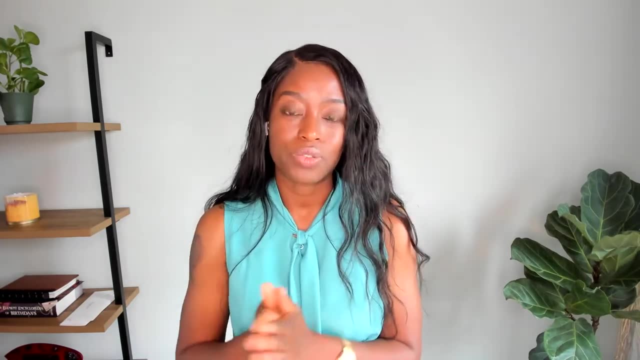 come and watch your kids- and i guess right now i'm specifically speaking to people that stay at home with their children. but imagine if you hired someone to come and stay with your kids. what would be the things that they do throughout the day? right, and i know that cleaning all day is not. 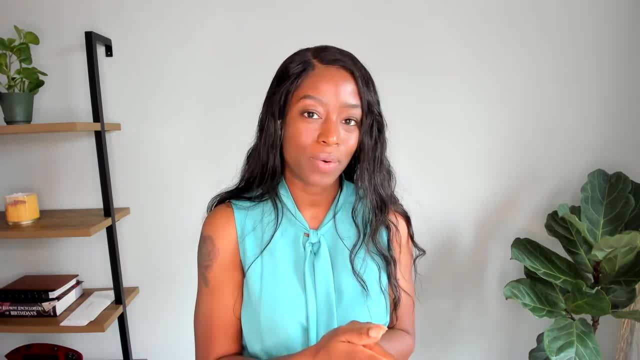 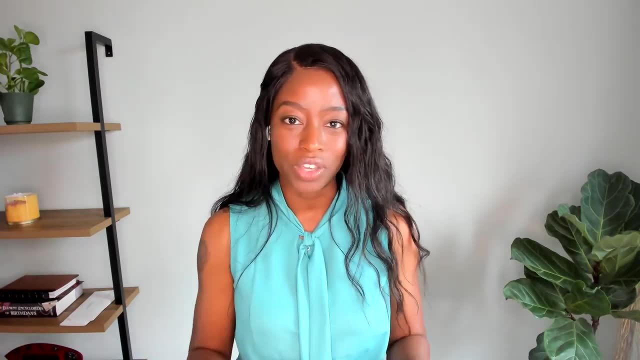 one. right, you have a cleaning person to do that and that should only take them maybe two hours, three hours depending on the size of your house. right? what should be getting done throughout the day? if you have your kids with you, there should be task activities. you know just what? don't do that. 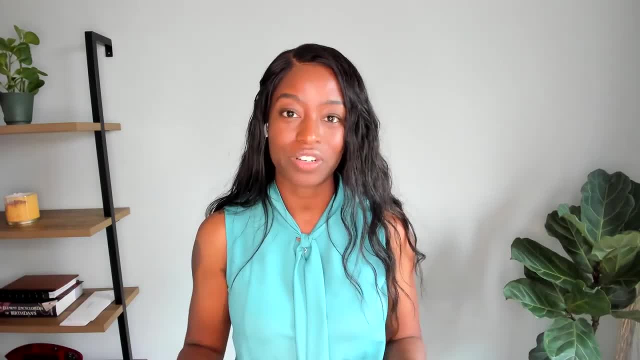 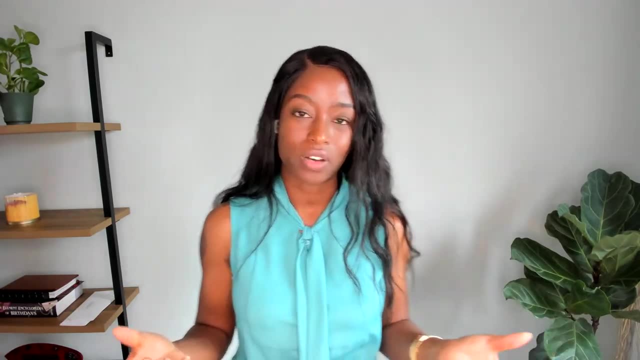 what would you hire someone to do with them? that's how I structured my day. again, you're cleaning all day long. no, that's not the right thing. you should be wrapping up. so let's say, go back to the whole breakfast example. right, we make breakfast, we eat, we wrap up. so what does the wrap up look for you? 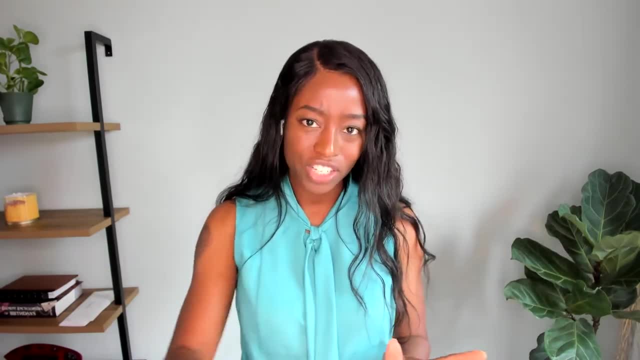 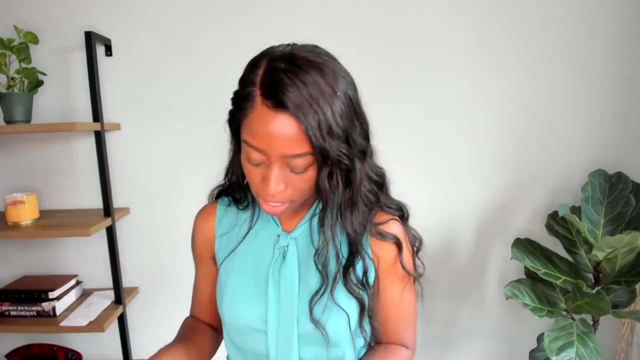 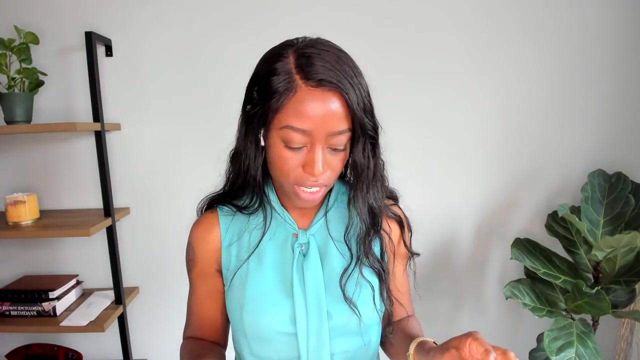 look like for you. excuse me, yikes, that should be when you clean up, and it shouldn't take you more than five or ten minutes to clean up for from breakfast. okay, this also. so there's actually two points I want to make here, which is that number one, in order for you to not be cleaning all, 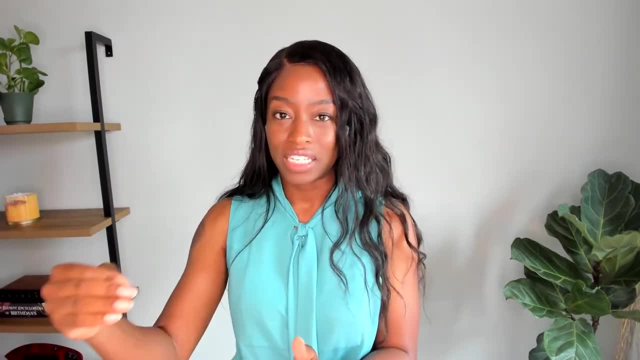 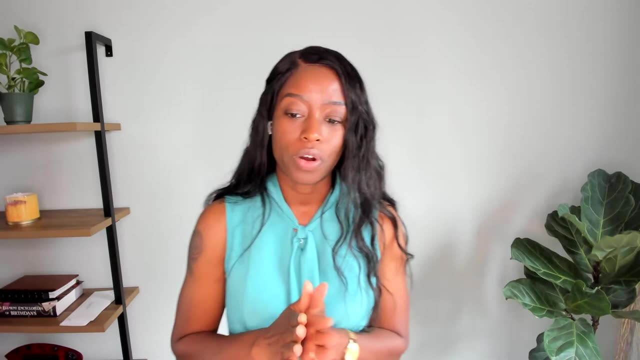 throughout the day. you need to know what your key tasks are that need to be done throughout the day so that everything flows, so to speak, okay. so for me, first thing in the morning, one of the key tasks that I need to do is: I need to know what my breakfast is, so I need to know what my 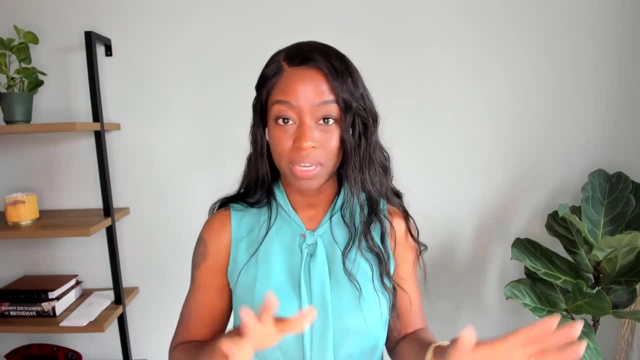 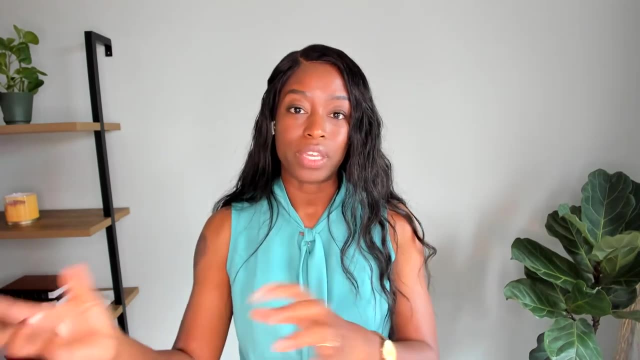 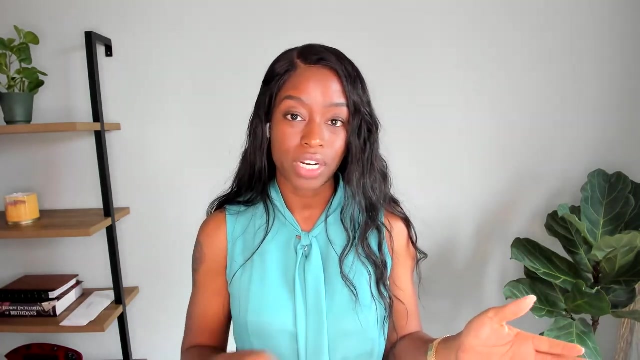 things that I have to do that, if not done, will cause basically a traffic jam throughout the day is: the dishwasher has to be emptied in the morning. that way we can easily put the dirty dishes into the dishwasher throughout the day and if at any point it does get full, we go ahead, run it, start. 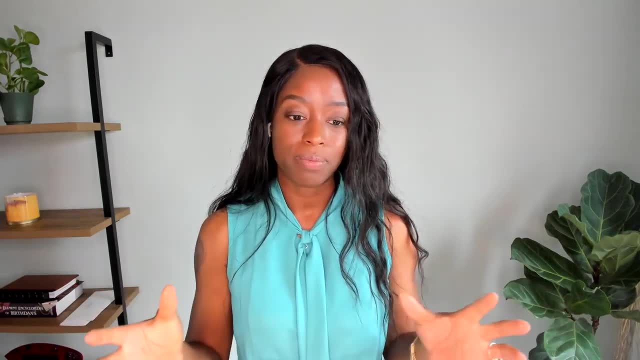 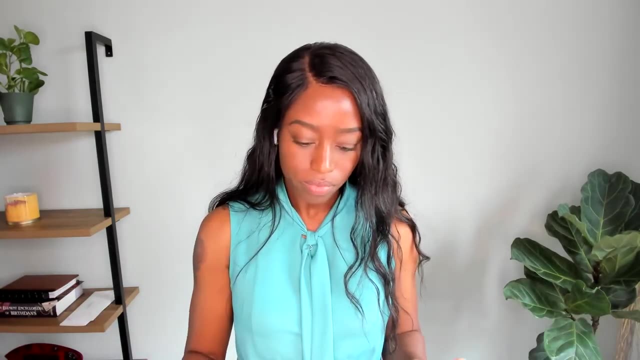 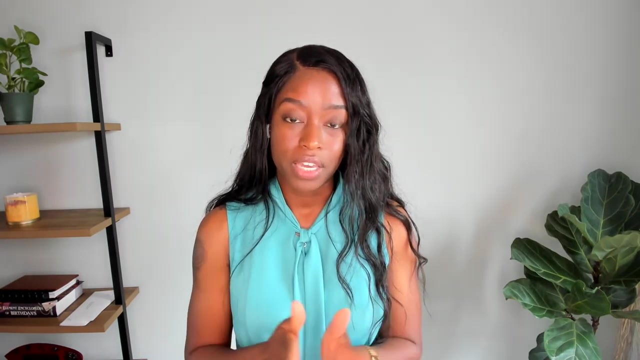 washing dishes or whatever it needs to be, but the goal is to try to keep the dishwasher empty enough to handle the dishes that we're going to be having throughout the day. all right, if you are trying to. I don't know, just know, yeah, laundry, same thing. right, I have a set time when I take. 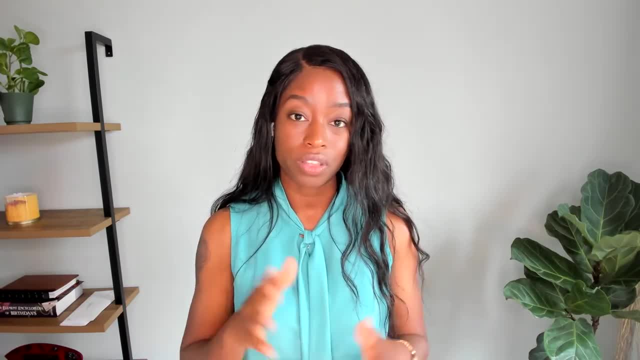 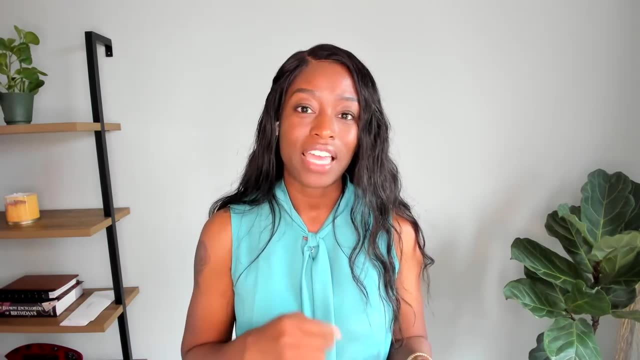 care the laundry right. so I started in the morning, right before the- the house starts jumping and all this stuff. I put the laundry into the washing machine. I started right then, and then my plan is to come back to it later. right, I'm not trying to like do all this in the middle of the day in. 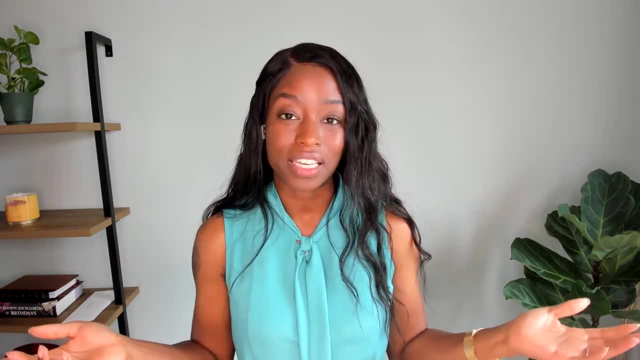 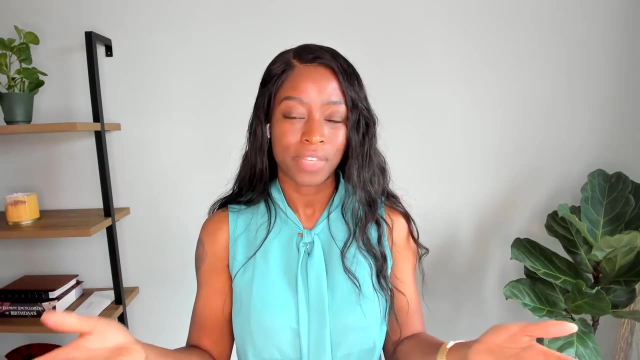 the middle of all the chaos or whatever you just it doesn't make any sense, right, I won't ever get it done. it's going to extend what should take me 30 minutes into a all-day thing, right, and you guys know exactly what I mean. like certain tasks, it really it doesn't take that long, it's just that. 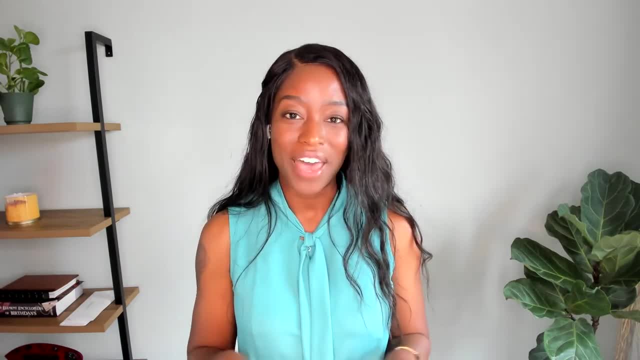 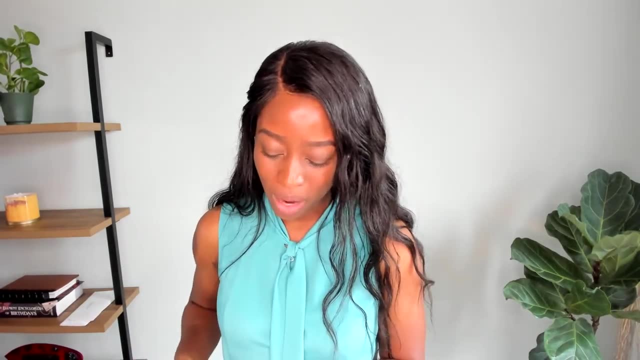 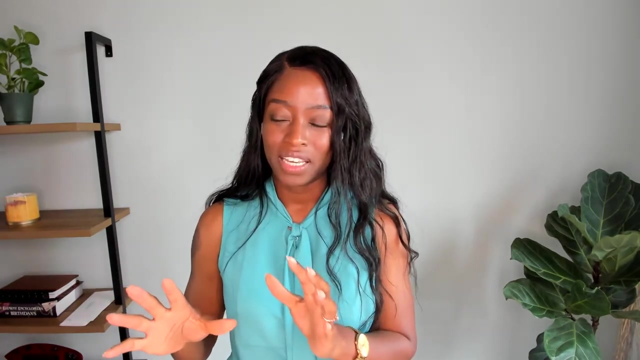 you're doing at the absolute worst, most inconvenient time ever, right? so just stop doing that. you're literally making your life harder than it has to be, and I want to basically go off on a tangent a bit, because you have to be able to do a lot of things, and you have to be able to do a lot of things. 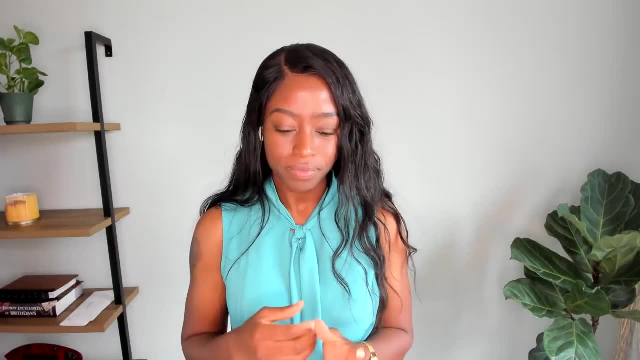 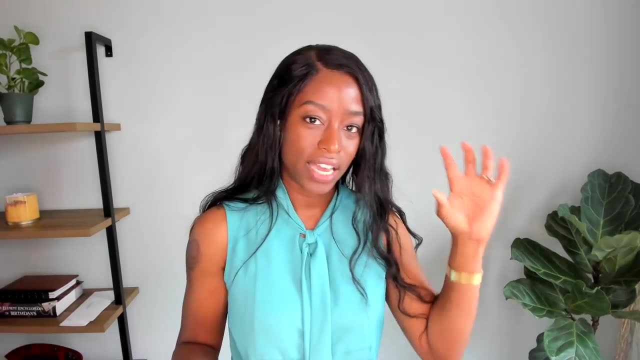 and you have to also look at people that work nine to five. right, a person that works nine to five, they come home and essentially they're going to do every single thing that someone's staying at home is trying to do throughout the day. but the person that works nine to five has a shorter chunk of. 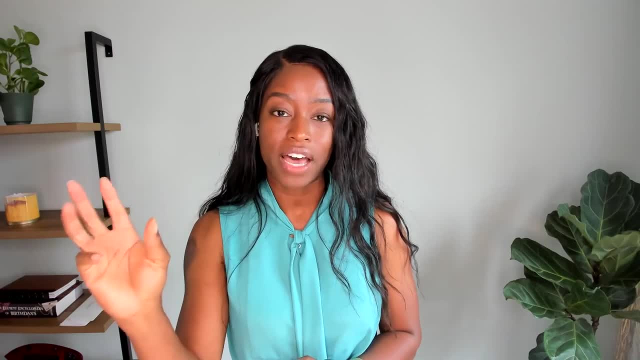 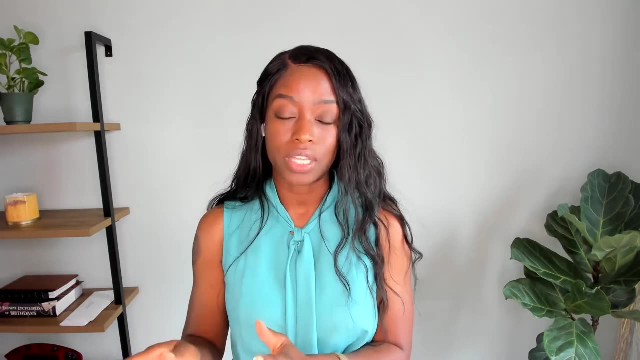 time that they need to do it within right. so they get home at five, so they have from 5 pm until, let's say, 10 pm to get all these things done right, and so that's what they do. well, now, when you stay at home with your kids, you're going to have to do a lot of things and you're going to 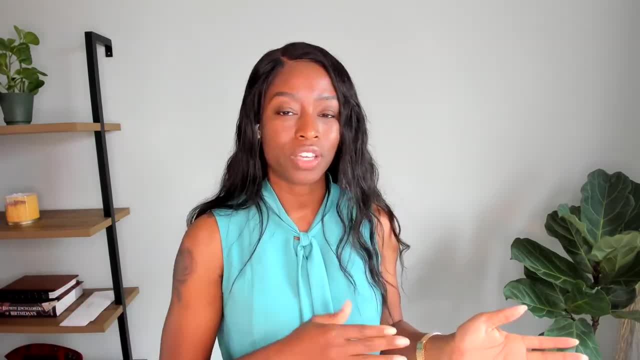 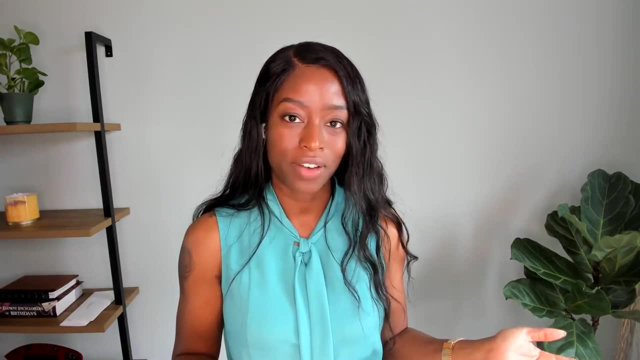 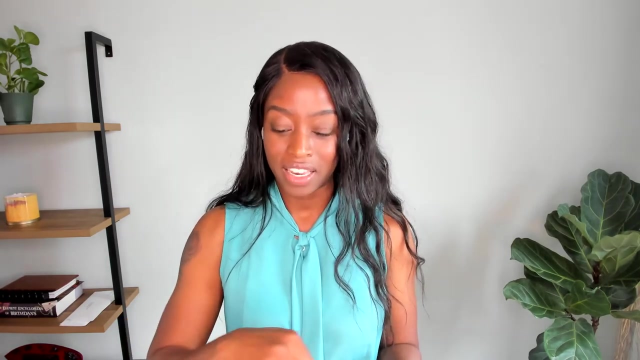 have all day. well, in your mind you're saying: you have all day, but you don't have all day. you should never think you have all day to do something, because then it does take all day, right? so let's go back to the beginning of this video, when I said that you know, hey, I've got to get this done in an 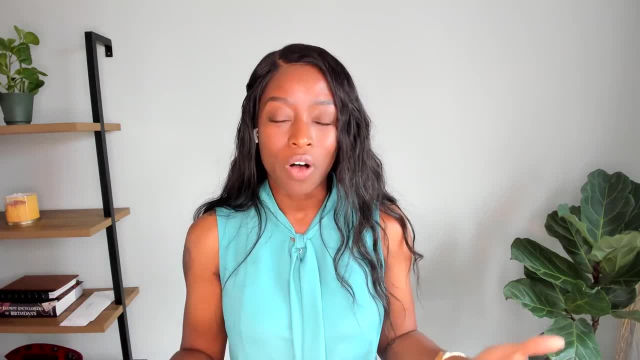 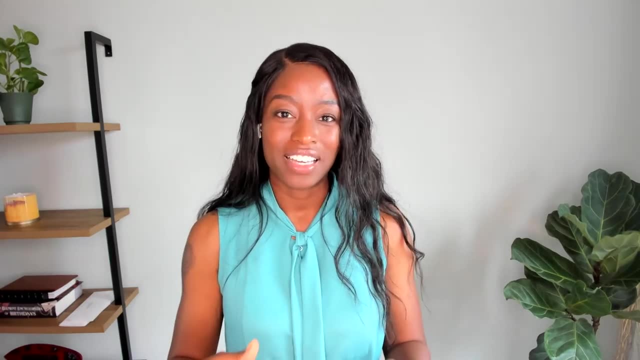 hour this video because I've got to go get my kids right. I don't have all day, so I have to do what I can do, as best as I can do it in the amount of time that I have, so that it gets done. it may not.